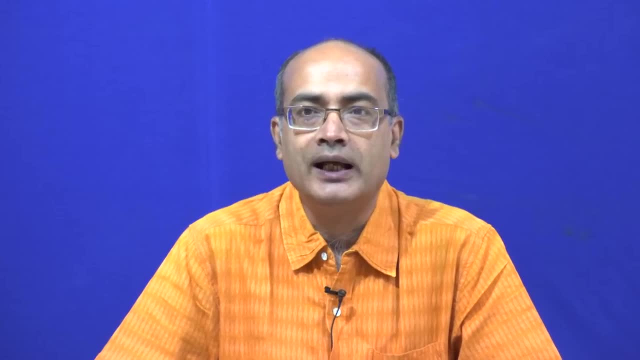 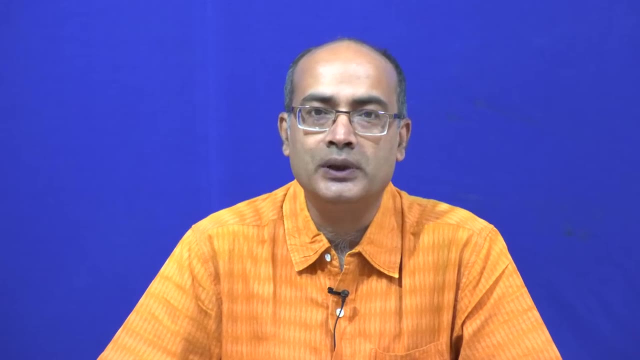 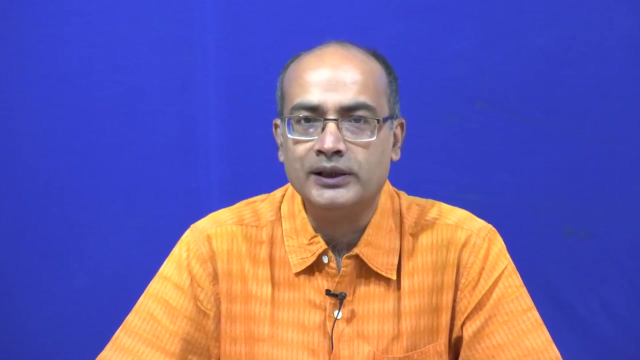 continue, continuously, keep on getting that feedback and that has become as an habit that I take it for granted. but when I am taking this online course, I could actually realize that that is not all the time which we can take for granted. we do not get the feedback that 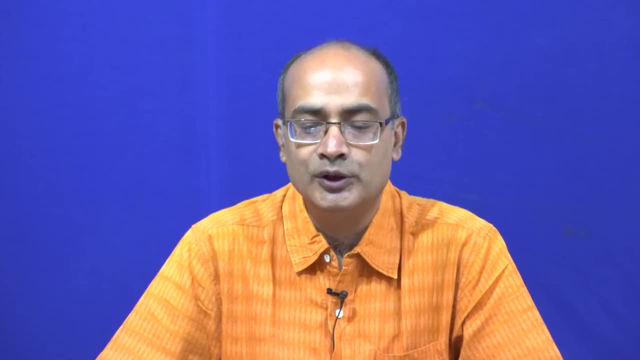 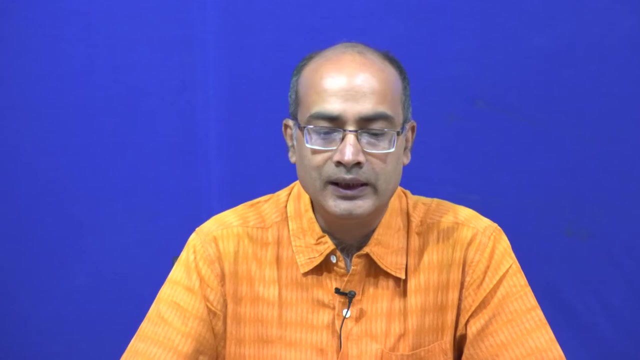 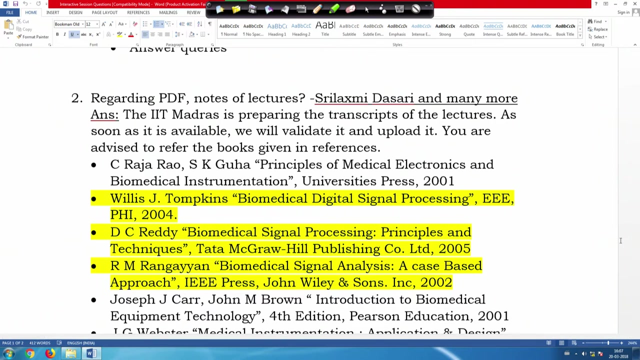 how the participants are feeling about that course. So I think it gives me an opportunity to interact with you and to reply to your queries. So that is the motive behind this interactive session. Next, I would like to go for the second question by Srilakshmi Dasari and many more people. 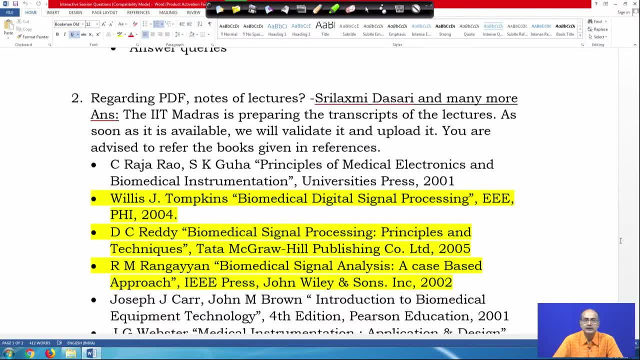 in the forum asked for that. this question that what about the notes of the lecture paper and pdf Now preparing the? the transcript is in the agenda of that NPTEL team and IIT madras. it is looking for it. they are in the process of preparing it. once that is available. 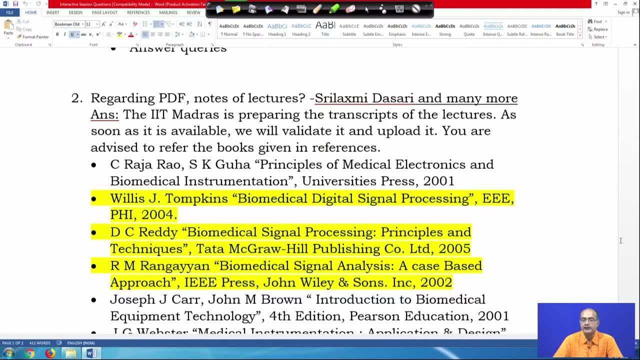 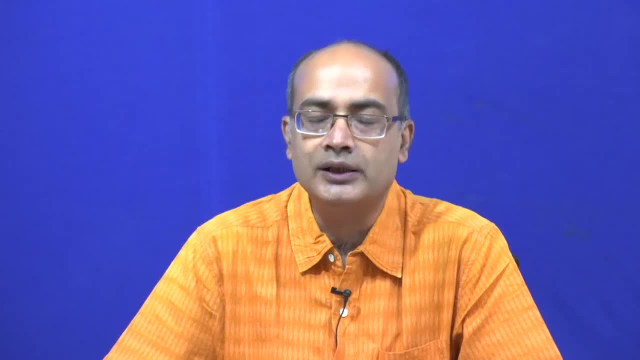 that would be shared with you. but till that time it is prepared, I think that we have enough material to go through. We have provided the class lecture or the video lecture. what we take that is just providing you a cursor to what to read and what is the sequence to maintain. And in the beginning, 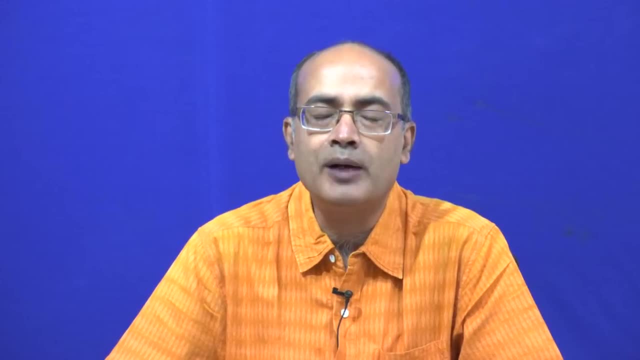 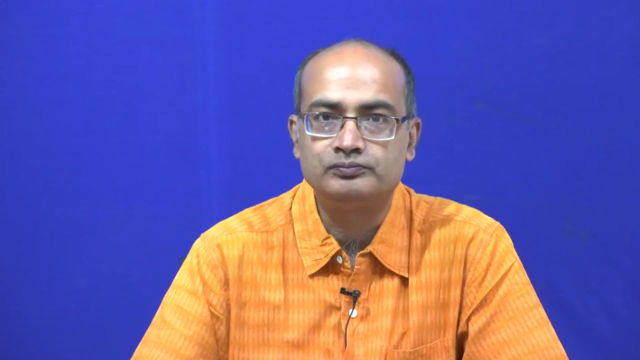 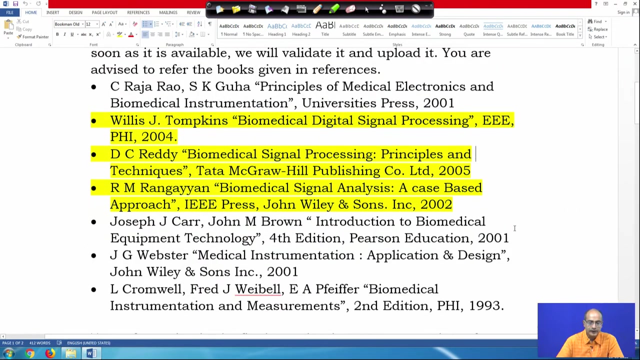 of the course. I have provided actually a number of references. when I went for that second phase also, I have provided actually the references and added one more name. I would like to go through them once more. So if you look at these courses, that out of them, that the three books we have highlighted- 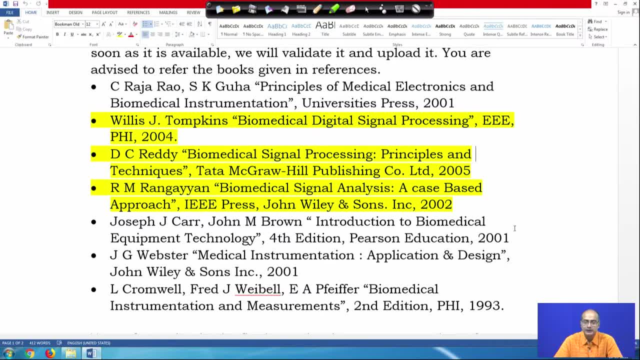 here all of them. they are on biomedical signal processing, that all three of them can actually be a text for these lecture course. So I think if you can get it from the library it would be the best. If you cannot get it, then I think you can buy it from the shop. we have the Indian edition. 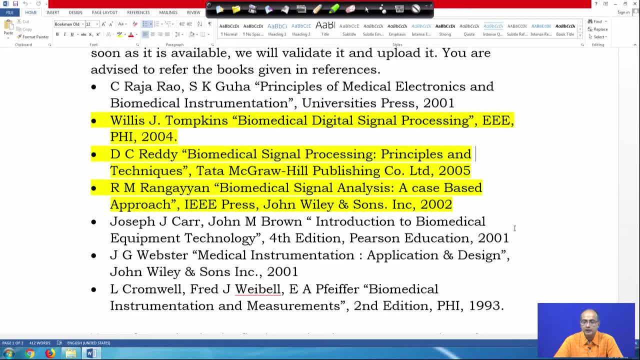 and the international edition. they are pretty affordable. So if you do not get them in the library, then I would suggest that you should try to get them. So one copy of one of these book which can actually provide you that the notes or what. 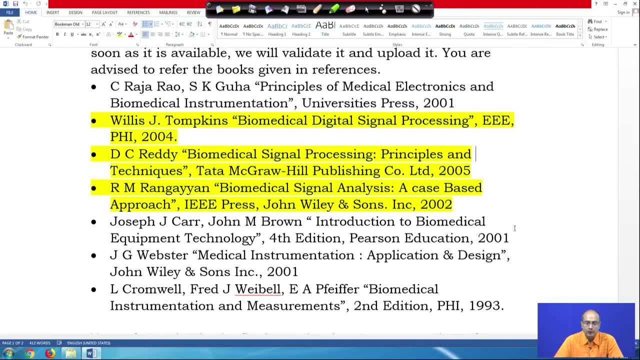 you are looking for The powerpoint presentation or the transcript. it can at best give you some bullet points. it cannot give you the whole story. So if you want to get the mastery over the subject, you have to go through some book and you can choose anything. 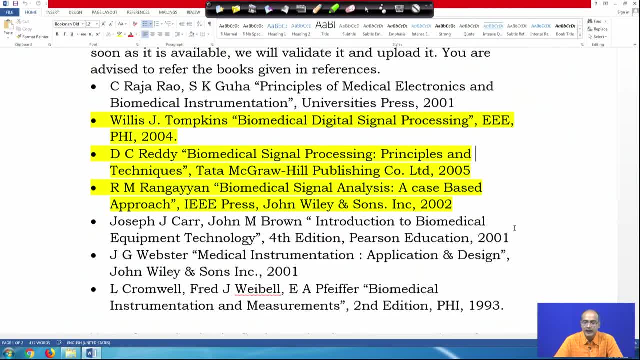 Any one of these book and the three books I have highlighted here- one by William J Tompkins, the other one is by D C Reddy and third one is by R M Rangayan- all three of them can serve the purpose of text and the other books they are. I would say they are the references. 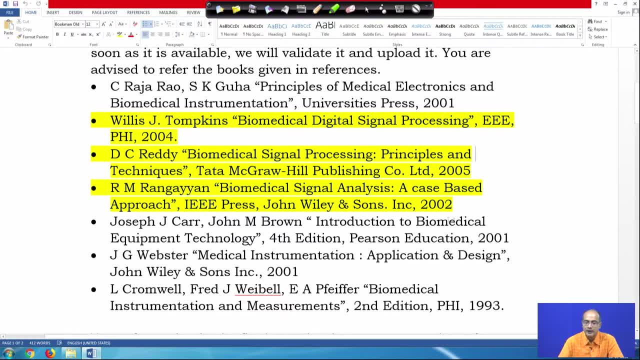 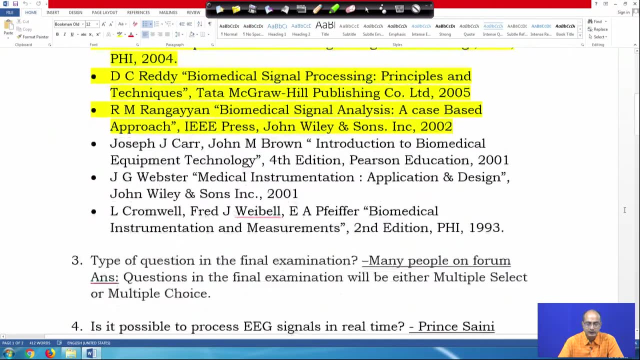 ok, So time to time they may be required. but if you have one of these three books- they are R M Rangayan, D C Reddy or that, Professor Tompkins- then I think your purpose would be solved. 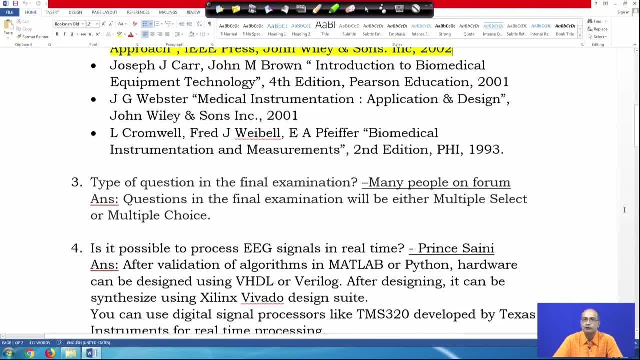 Next, I think many more people has asked in the forum as well as in that Google sheet, that what would be the type of questions in the final exam. It would be exactly similar to the questions you are getting in the assignment. In the assignment you are given number of questions and all of them they are multiple. 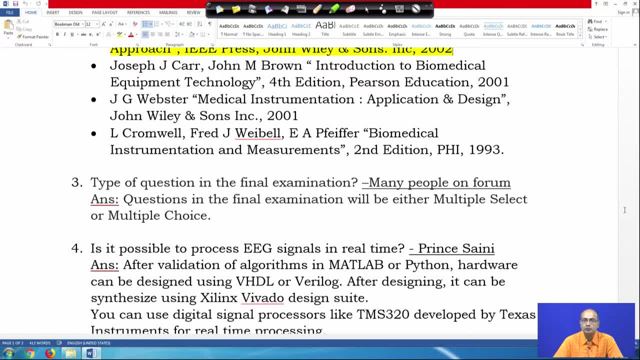 selection or multiple choice, So you will get the similar kind of questions. so either from your knowledge, you need to select one or multiple of them, Ok, Or sometimes you need to do some small computation using calculator to get the right number before you make the selection. 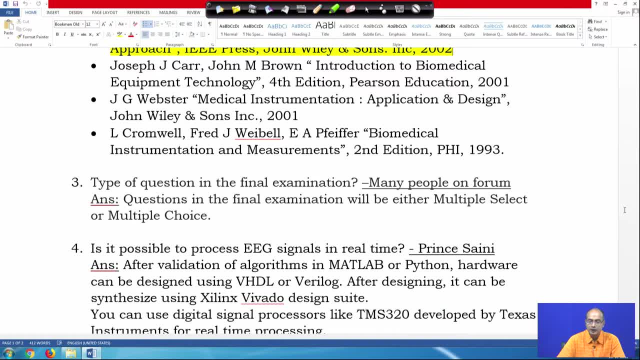 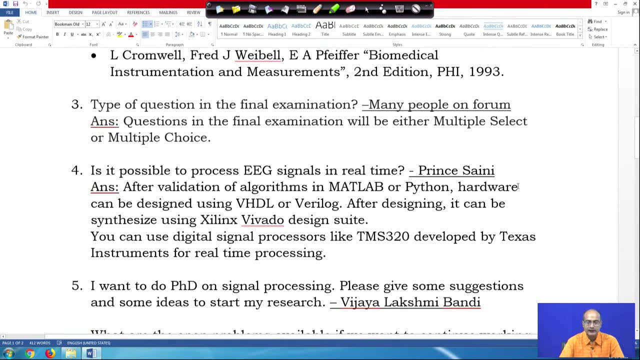 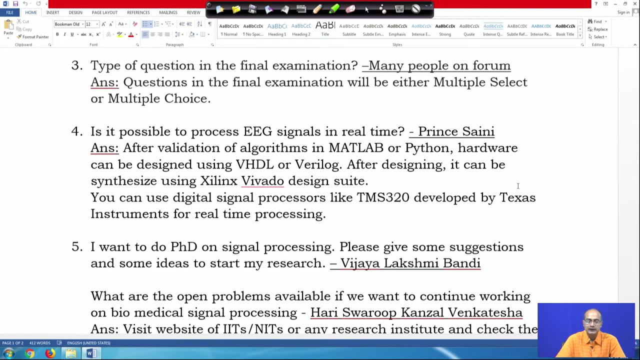 So that would be about the final exam. I am not taking the name of the that. the participant who has asked these questions, because I think there are a huge number of participant asked the same question. Next question: that from Prince Haini. the fourth question is that: is it possible to? 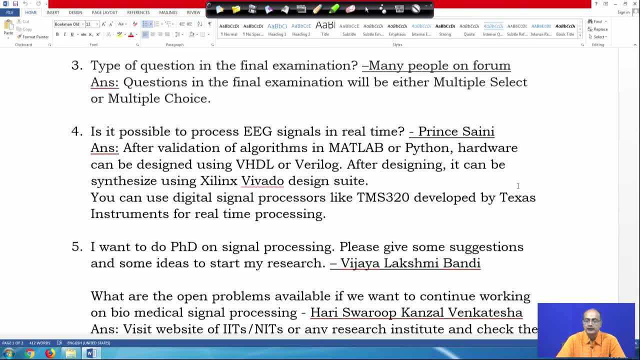 process: EEG signal in real time. Yes, it is possible that there are number of techniques actually to do it. First of all, from week 9th, when we are doing the that tutorial In many place actually that I pointed out there that please look the that filters what. 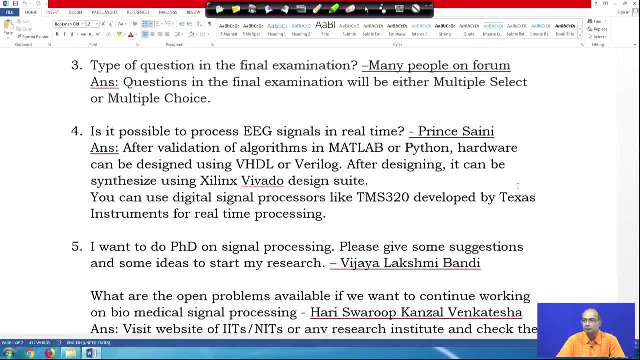 is used. they are integer filters. So you know that if you try to do some addition or multiplication that in your computer, that if it is integer it takes less time. if you want to have that, a silicon implementation of the same, It takes less space and less actually that the computation. 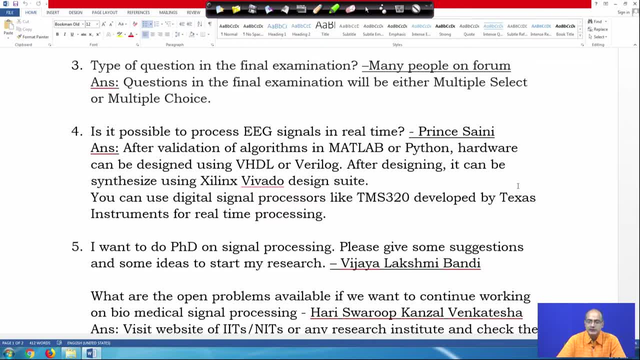 So if you can do the processing with integer number, that would be the best. The first step towards it is first you implement it in MATLAB or Python. So check the functionality of it and you get an idea about that, how much time it takes. Next you can choose an appropriate platform. 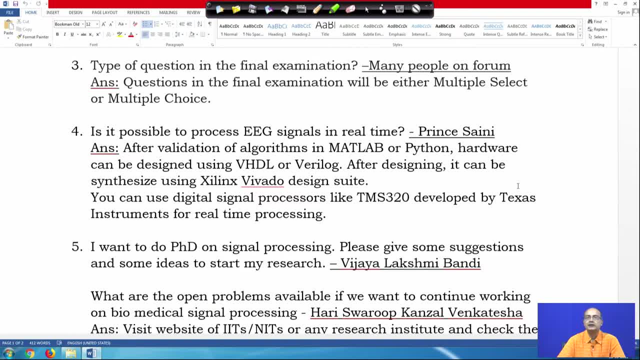 It could be an embedded processor like ARM, or it could be that a, actually that FPGA for which you need to do that VHDL programming, or it could be a DSP like TMS320, from text as instruments for real time processing. So, depending on that, how much computation you need? or, to be more precise, 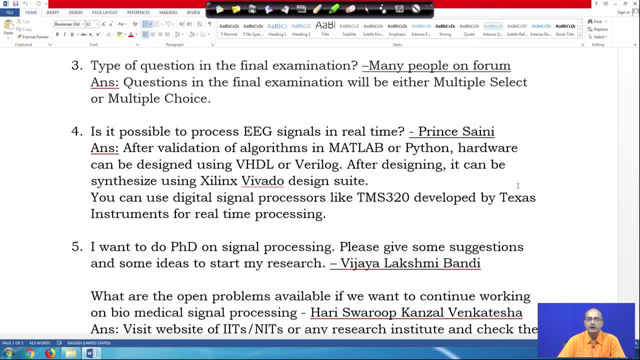 So it depends on that. That when you are talking about real time, that means you have a constant over the time, over processing. that may be you can just wait for the next sample to arrive. So within that you need to compute the that whole process and be ready to take the next. 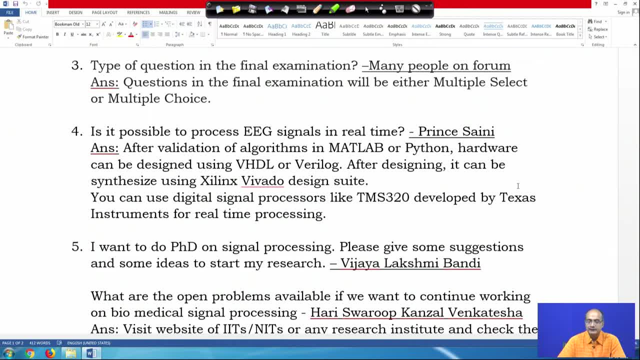 sample. So for that you have to choose appropriately that, what platform you would use. So that is the first step, The second step, The third step, The fourth step, The fifth take And if I want to actually name one of the real time application that nowadays, those 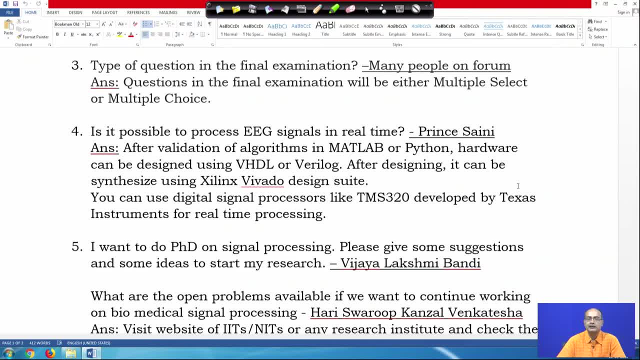 the pacemakers are there. They are actually supposed to give a bit, because the hard bit, the signal, comes from the SNO. it may not be coming all the time, So pacemaker is supposed to provide that bit. So that is the first step. 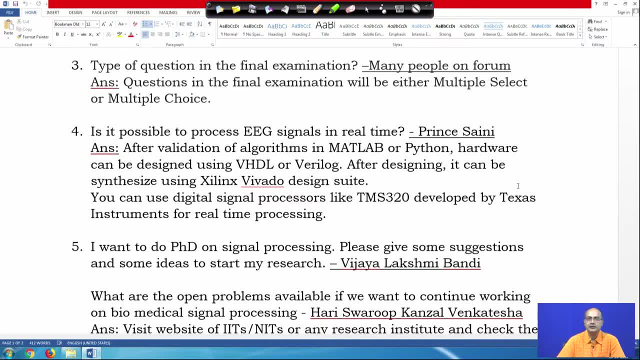 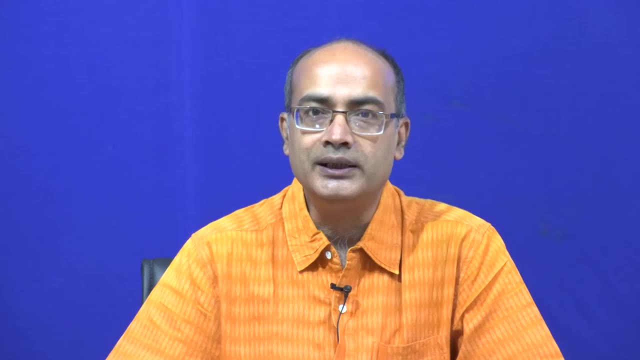 The last step, The fourth step. Next Now initial the prototypes, or the initial days, the first generation. the pacemakers used to all the time provide that bit. So whether SA node is working or not, it is continuously working. Now the effect of it is that it would need actually a bulky that battery and still the 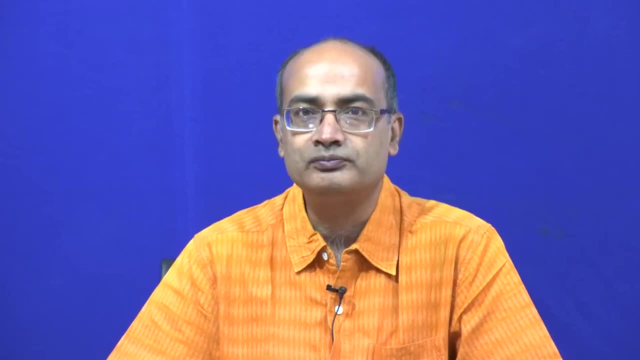 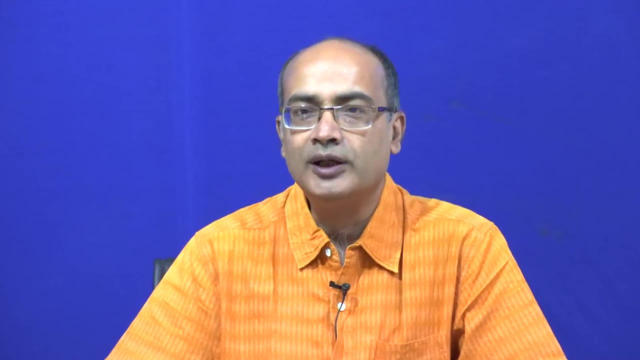 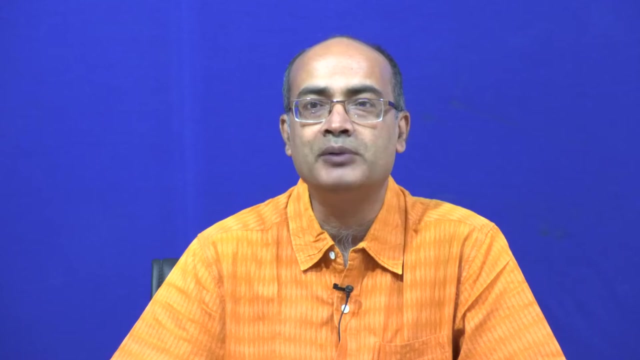 battery will get drained because it is working all the time. So after that that the researchers- they found that SA node is not that bad here. some problem is there for a particular patient. So they are not working all the time but most of the time they work. 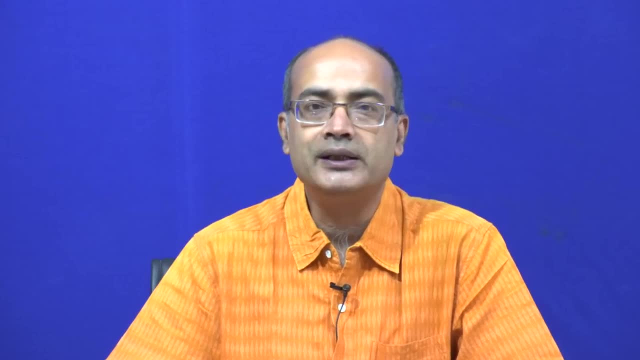 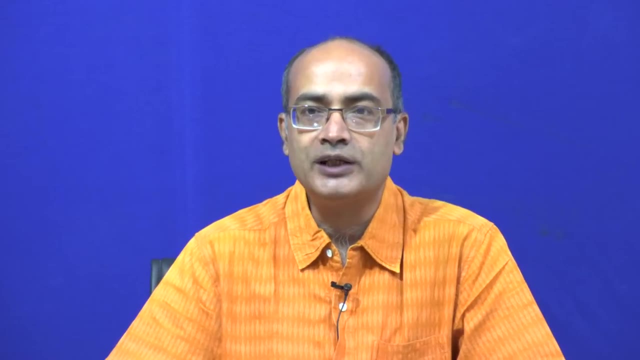 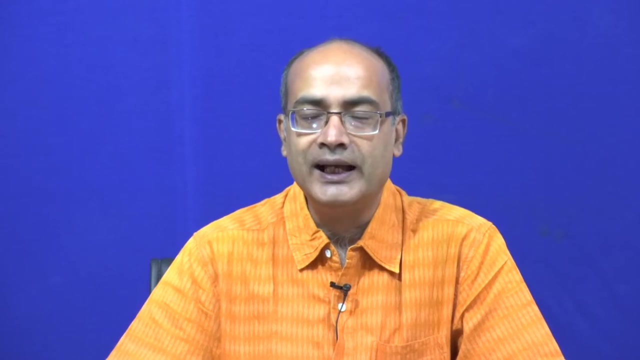 Sometime for some problem. they do not actually give the bit in time and the patient suffers for that. So they made the pacemaker so intelligent That it will work. So it should be waiting for the SA node to act and if they find that SA node has missed. 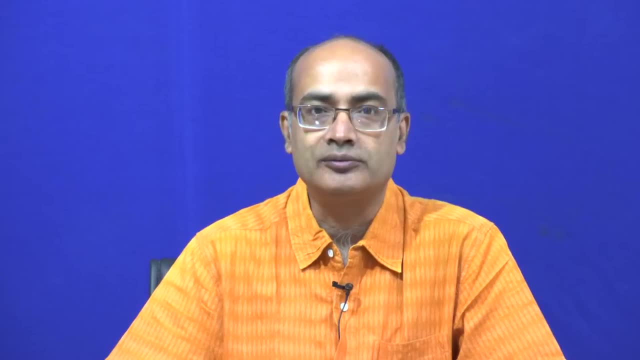 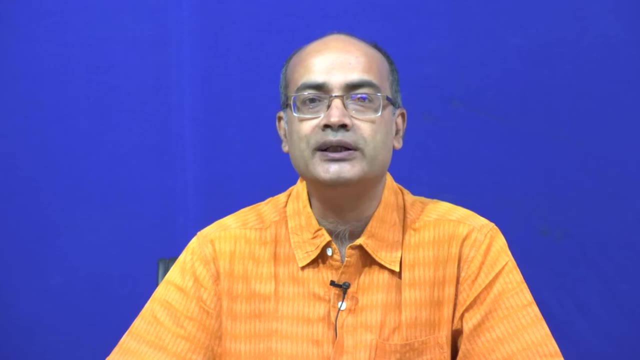 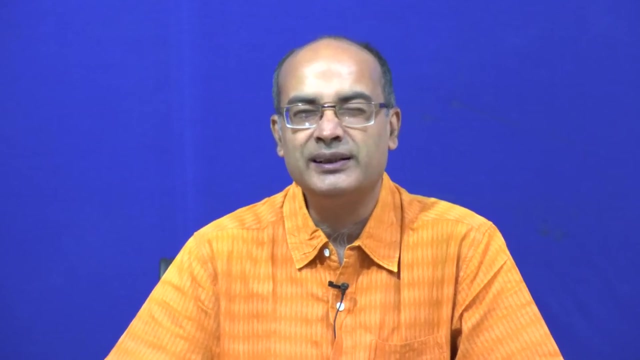 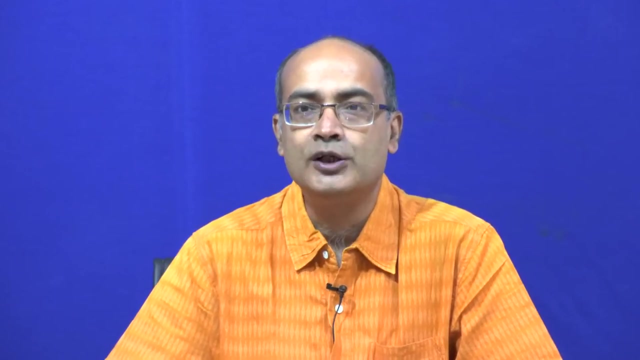 the bit, then it will take over and still it will again keep and watch whether the SA node have actually taken up its job again. If the SA node again started giving the bit, then there is a chance that you can have. actually is that ectopic bit because 2 signals or 2 commands are coming. 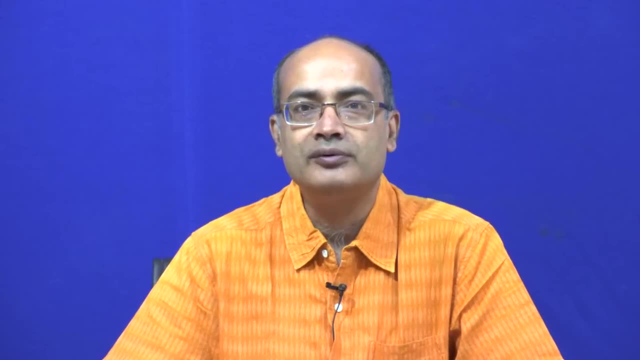 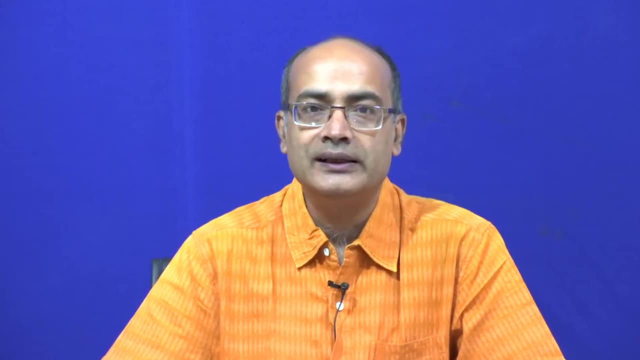 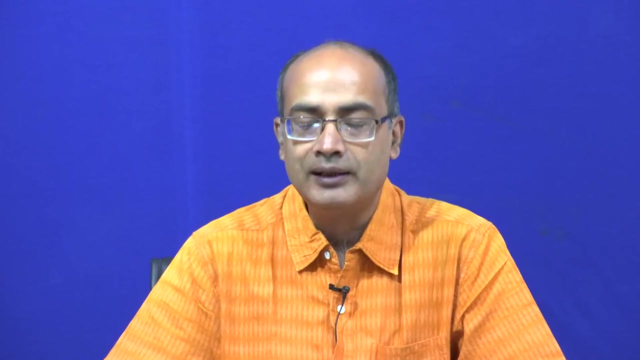 So the pacemaker again will take itself in sleep mode or listening mode and allow the SA node to work in a normal way. So that is completely in real time. it does the job. So there are lot of applications for which the biomedical signal processing you will. 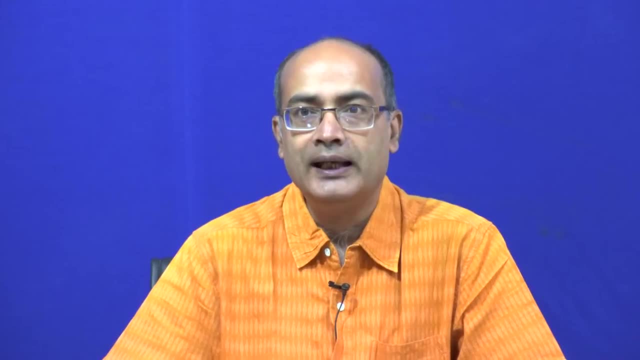 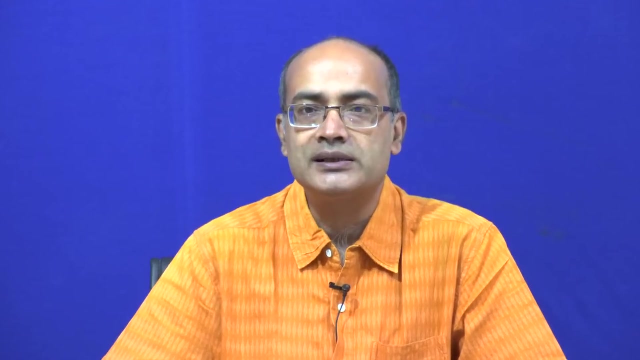 find that it works in real time. It goes from sleep mode to listening mode, So the pacemaker take itself in sleep mode frequently And I would say that it is not a that big a challenge because that if you look at the signals, the frequency of the signal is much less compared to the that the communication. 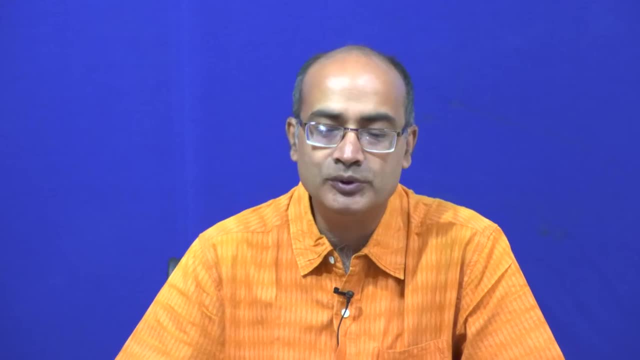 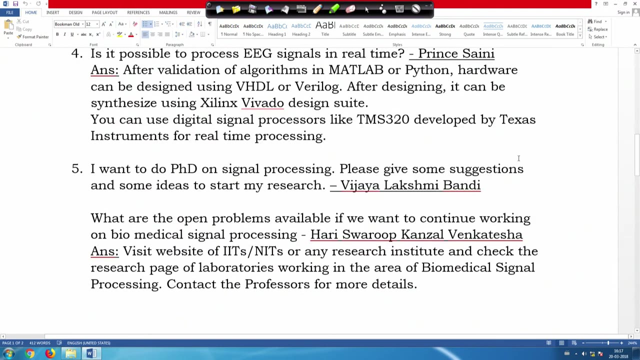 signals. So it is highly possible to actually that process them in real time and it is done in real application. Next question: I get that that we have clubbed actually number of questions, one from Vijayalakshmi Bandi. that question is: I want to do PhD on signal processing. please give some suggestion. 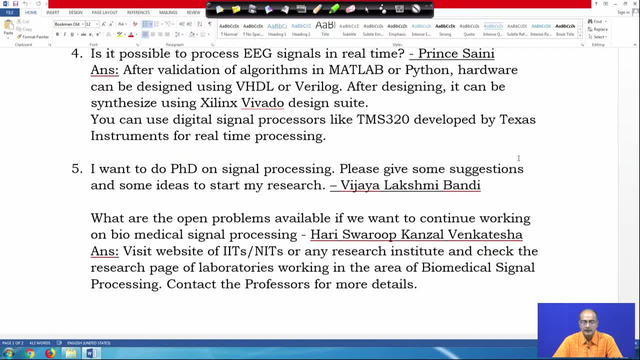 and some idea to start my research. That next, that along with that, in similar line, what are the open problems available if we want to continue working on biomedical signal processing? This question has come from Harish Haroop and that I would say that such question should. 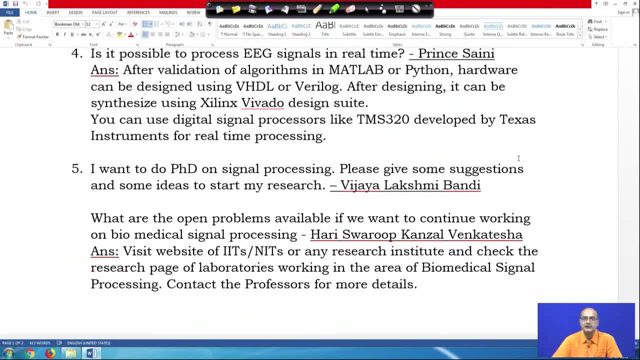 be taken one on one basis. That means you should ask the question on personal level to any faculty. you can go through the web page of IITs or NITs If what you find out that whose interest are actually matching with yours, there are number. 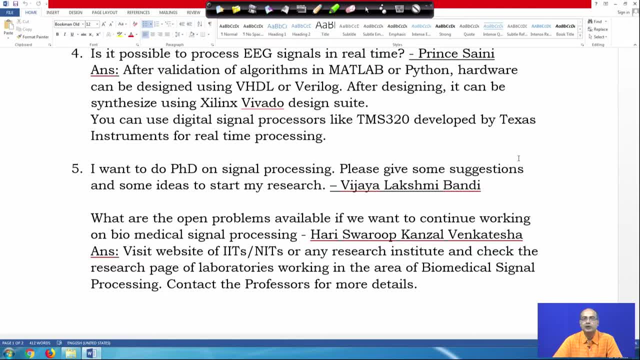 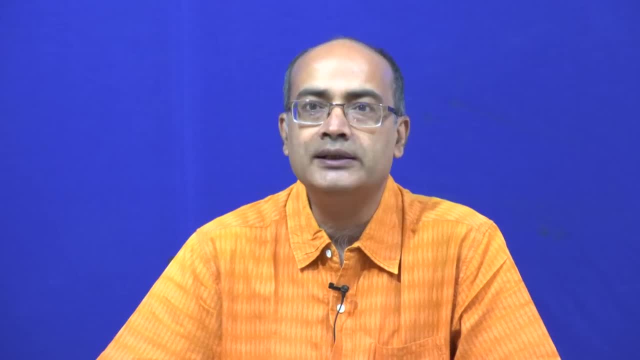 of actually good researchers in India who are working in biomedical signal processing at present. I look more towards that, that image processing, medical image processing rather than the signal processing. Anyway, you can contact in any one of them and it would be the best to get the suggestion. 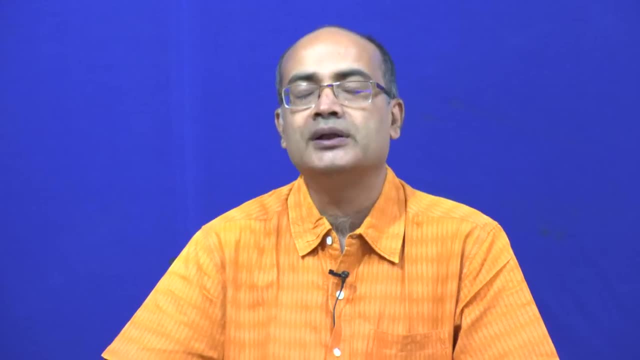 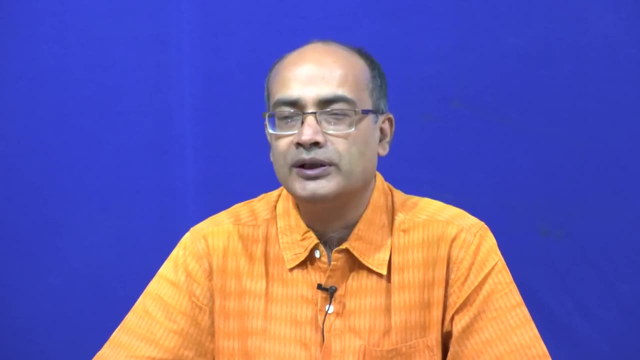 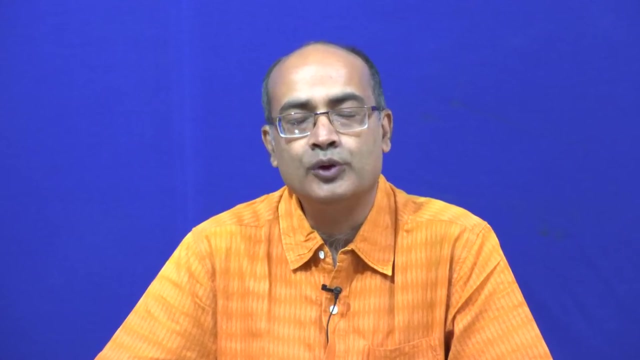 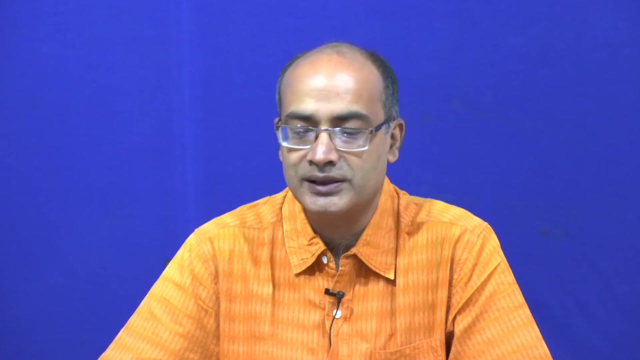 from them And there are number of open problems and they are working on them and all of them could be very good use for the mankind and that it can help to the people of our country as well as throughout the world. And one more point: that all such applications they are for the peaceful purpose which we 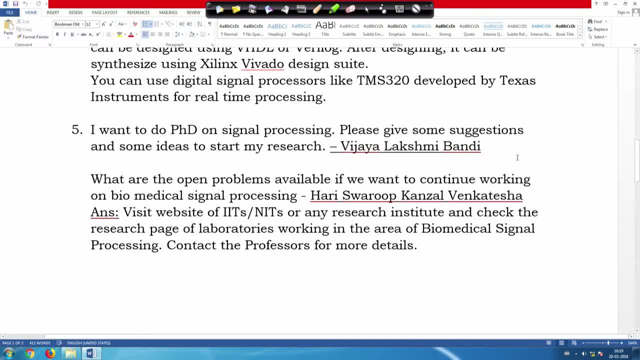 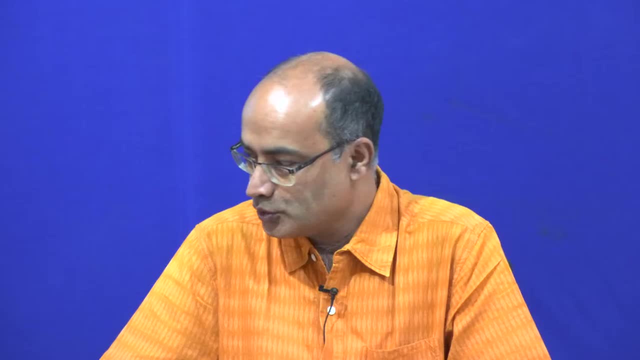 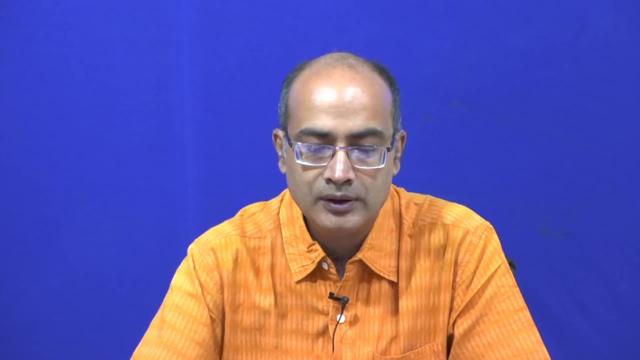 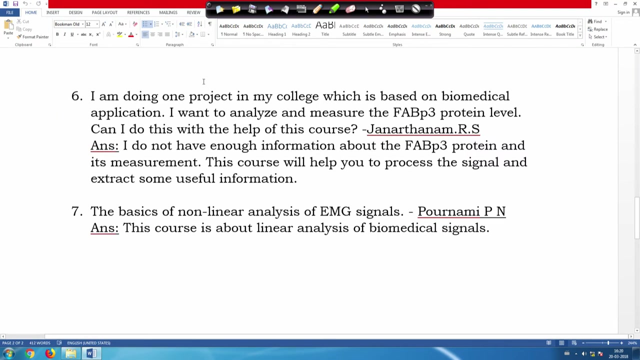 sometimes we miss for the other technology. ok, So you are most welcome to do the research, but I think such question should be asked in person to one expert with whom you would like to work. So ok, we have some more questions already given in the Google sheet. 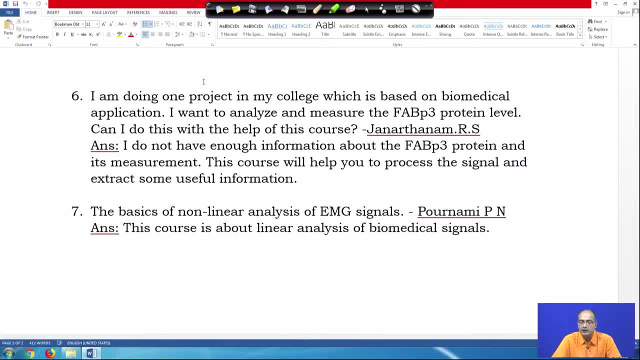 From: Ok, I am doing one project in my college. what is based on biomedical application? I want to analyze and measure FAB p3 protein level. can I do this with the help of this course? I am very sorry, I do not know enough about that FAB p3 protein. 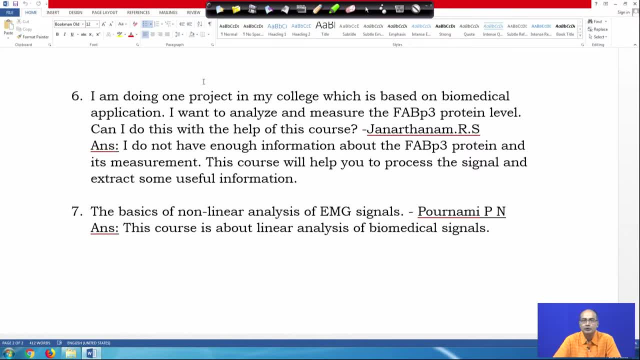 Now, if you share some information that how it works or so, Then we can try. so this course is primarily for that: biomedical signals and how that signal can reveal the internal physiological process going in the body and thereby you can get that whether those physiological process they are going in a normal way as they are expected. 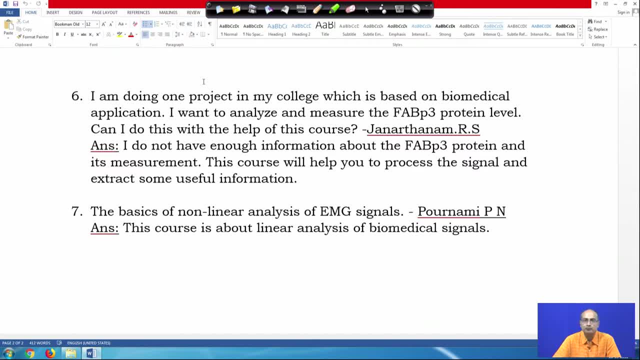 to go or they are facing some problem. Ok, So sorry, I could not help you at this moment. Next question is the basics of non-linear analysis of EMG signal. This question has come from Purnima PN In this course. primarily we are looking for the that linear actually processes linear. 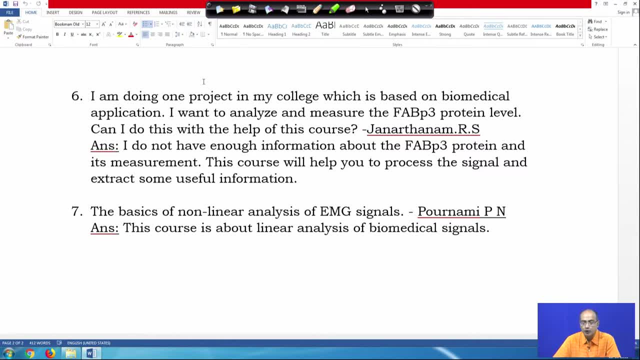 signal processing, I would say Ok, And we have not gone for the non-linear models. however, if you have any non-linear model in mind, yes, they can be tried. we will have used them for different kind of biomedical signal, because linear signals always cannot actually express the complexity of that signal. 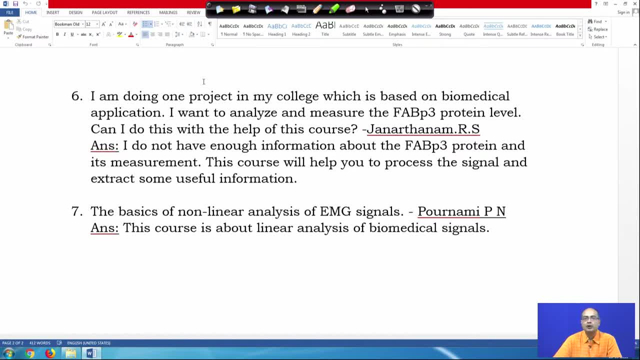 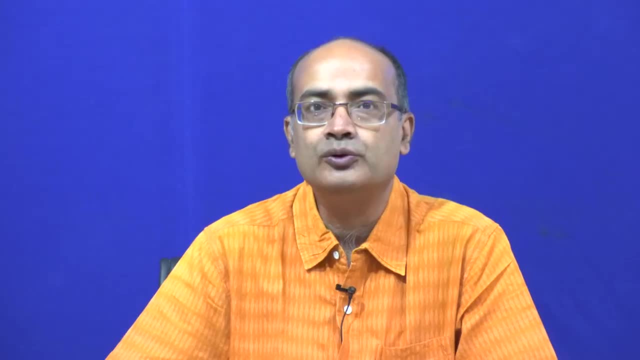 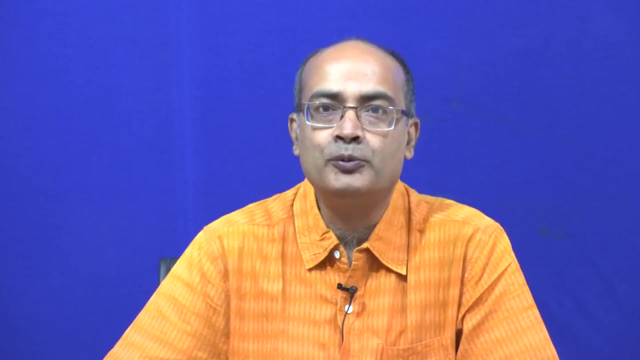 The other way you can look at it, that all these signals, they are basically non-stationary in nature. So another alternative to the non-linear system is that linear time invariant systems. that is also another alternative you may explore. however, in this course we cannot go up to. 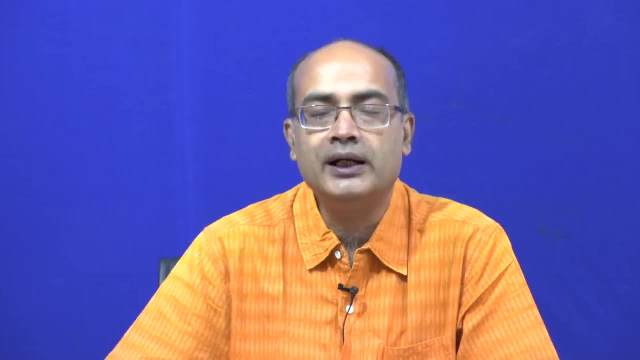 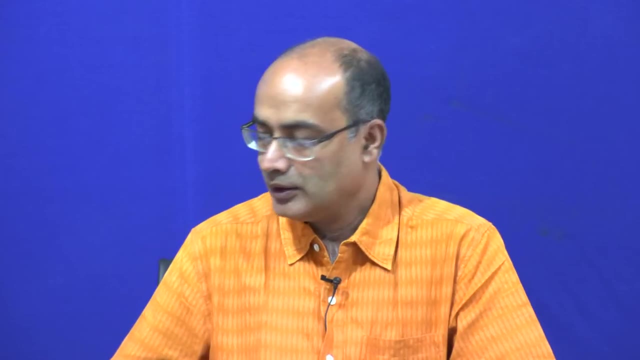 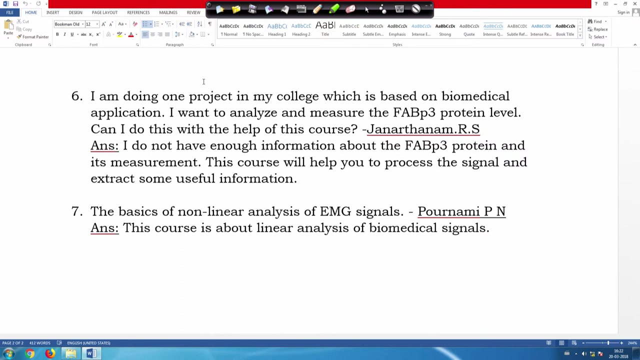 that. so we restrict ourselves from within the the boundary of linear signal processing. Now, Ok, So let us. we got just one more recent question for by Sivamshu Tyagi. the question is: what makes biomedical signal analysis more difficult or challenging than other physical signal? 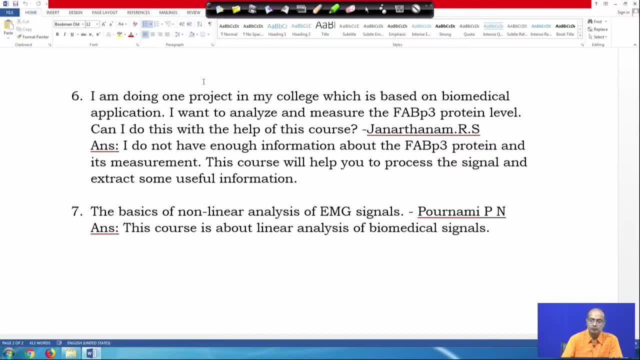 analysis. So it is a very good question that, if you look at that, the signal analysis, We model it as a linear way. however, it could be non-linear at times and there are many challenging applications like. one simple application you can look at is the ADSL modem. that is, we. 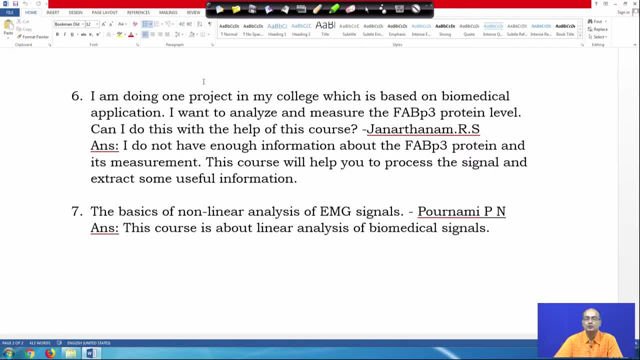 call the broadband access technology, those who still have that, the wired telephones. we know that we can get a high data rate within that And the principle of it is very interesting that only up to 8 kilohertz- that is the bandwidth that we are using for the voice actually speech, within that that we have the signal beyond. 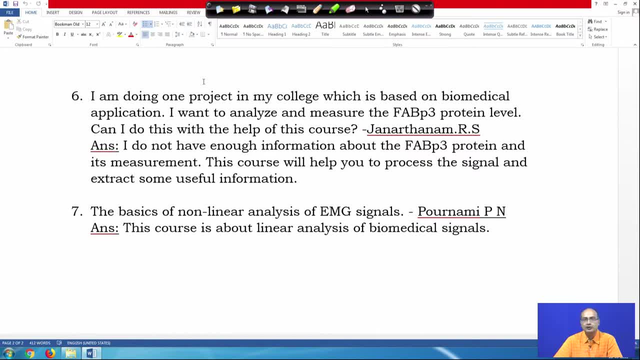 that there is a huge bandwidth for that cable, but that bandwidth is not utilized, primarily for the reason that that part is very unreliable, In the sense that from one actually cable to the other, that in between, that means the from your actually instrument to the, that the exchange in between, the pathway, that the 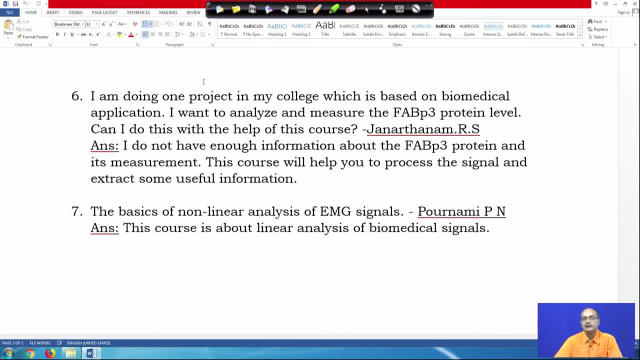 channels are there, that is, the cable connections. they are not same and because of that their attenuation characteristics in different frequencies are different, So you cannot standardize them. in case of ADSL modem, what they do, they break that into multiple actually channels and check all of them and find out that which are reliable. 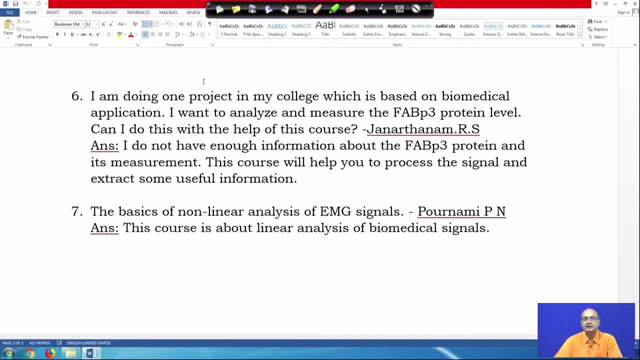 or strong in terms of the SNR, and they pump the data within that and they dynamically actually look at that, because this characteristics also changes with time. So you know that there is a pattern that how the modulation would be done. those things are known. but in case of the biomedical signal processing, the main challenge is that 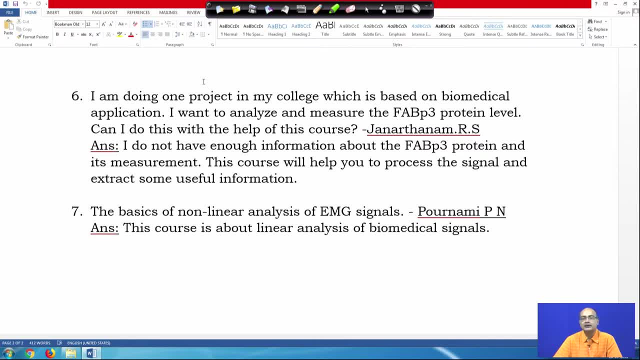 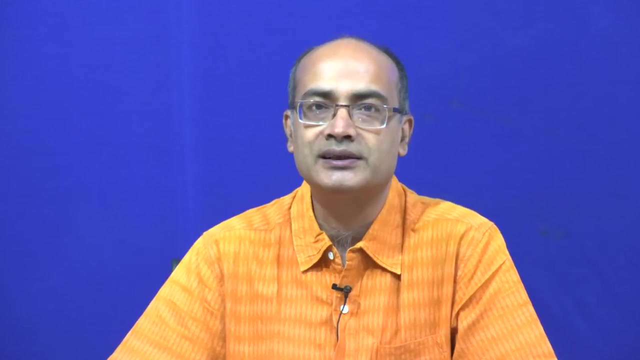 the source is actually that the human physiology or the human body, and each one of us is little different from the other, So signals are changing, though the overall pattern may look to be similar, So treating them becomes more difficult and the variation is more. in that case, and 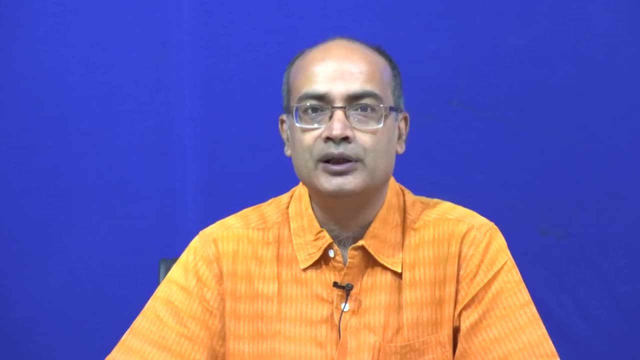 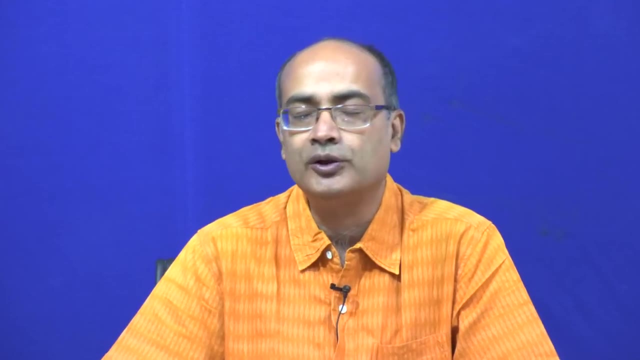 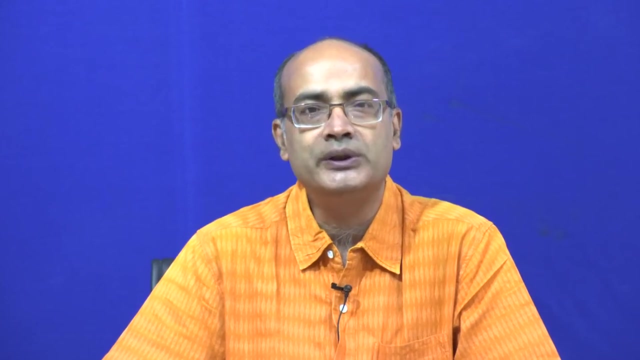 what I would say? that there is continuous variation. you will get a spectrum of people whom we can tell that they are actually normal. if you go to the doctor, they will tell: yes, you may find it actually different from other people, but it is within the normal range. 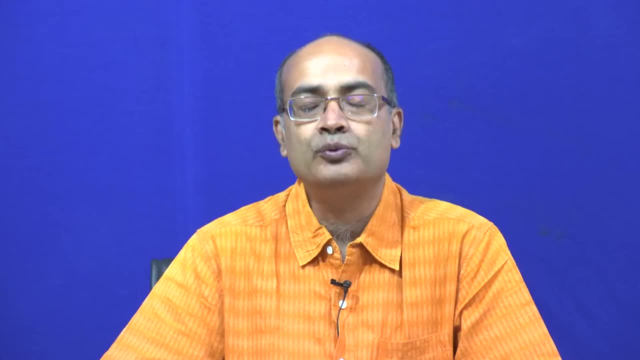 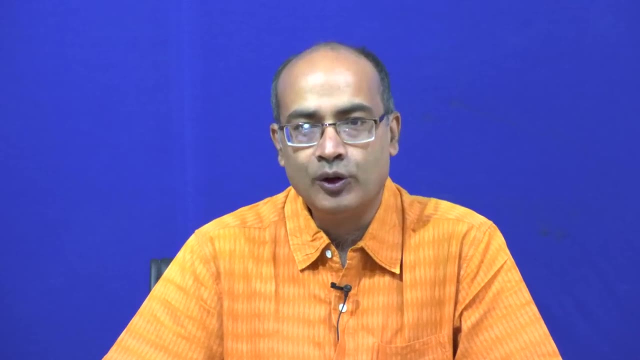 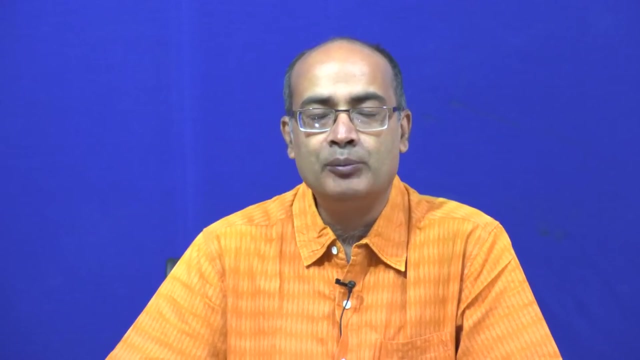 The resent same way that those who are. we call that having abnormality or pathogenic signature. there also a lot of variations are there. So that makes actually biomedical signal processing more challenging. but the good part of it, that biomedical signal, the frequencies are much low. 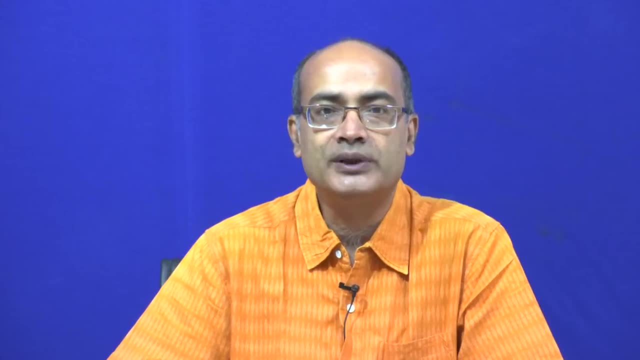 So that makes the thing easier in terms of the real time implementation. However, for the analysis of bisso- 좋아요, кстати, we are thunder at 8.50.. However, for the analysis of the signal, it is not actually that easy and it is actually. 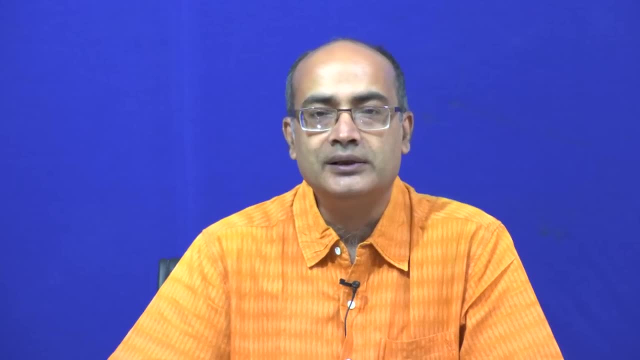 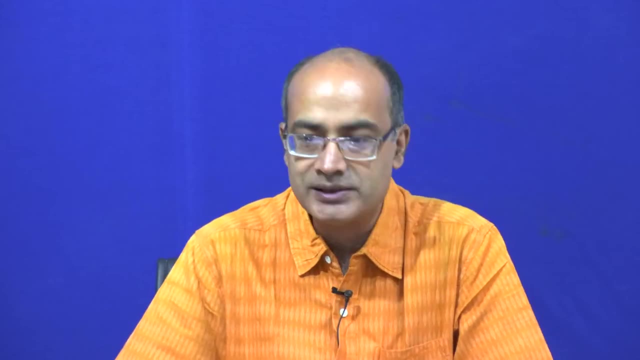 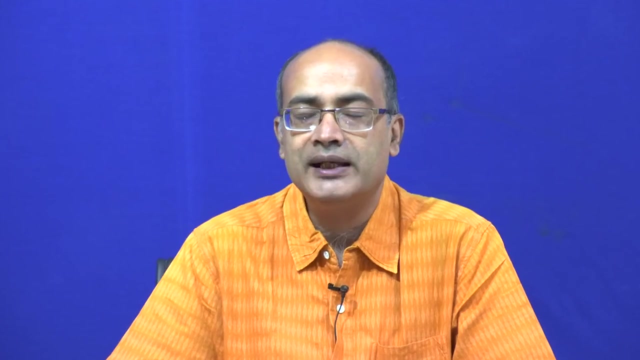 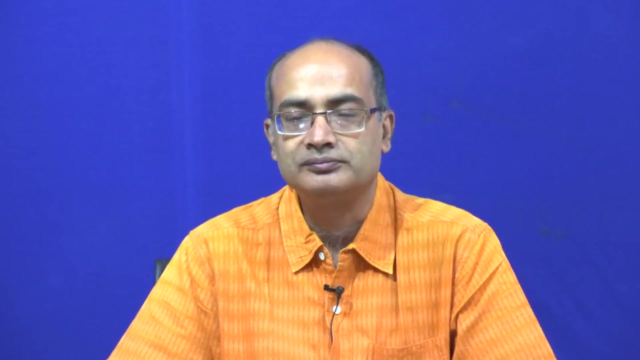 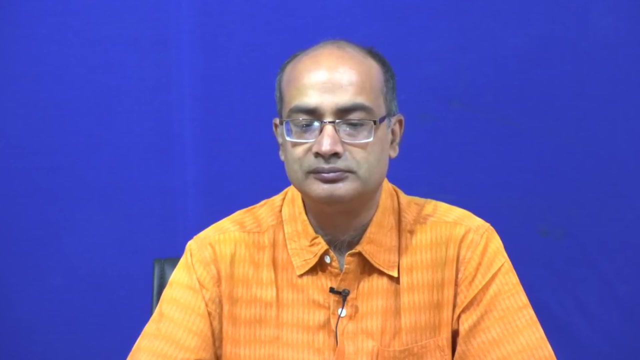 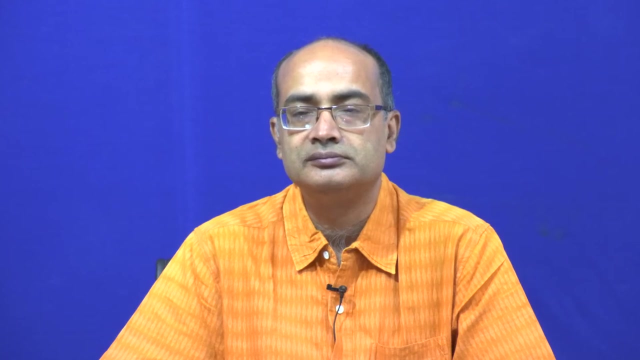 more difficult than the our. that communication signals. So these are the questions we have at this moment. If you have any other questions, you can just actually text it in the chat box and we would be ready to pick up those questions. Thank you for watching and I look forward to seeing you next week. 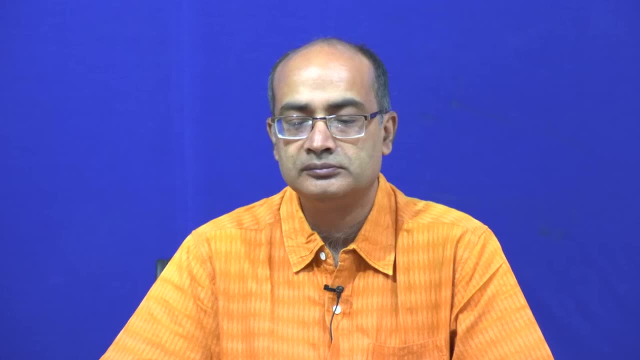 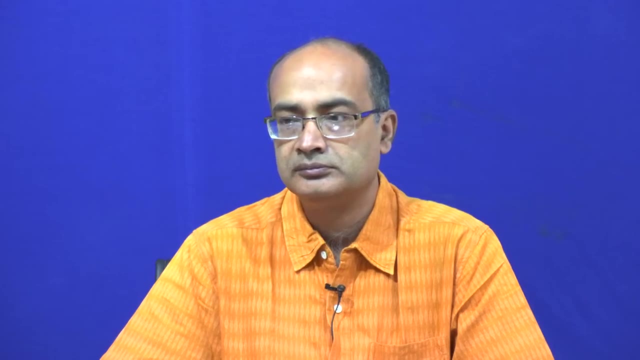 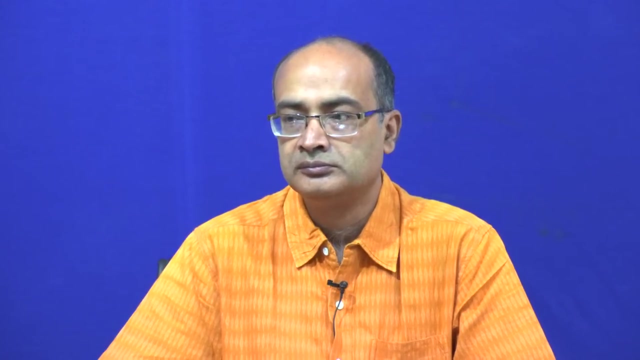 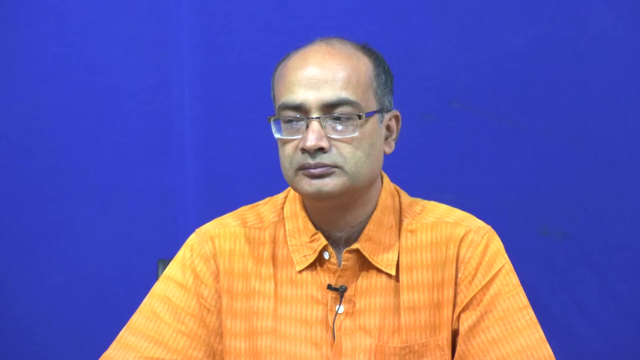 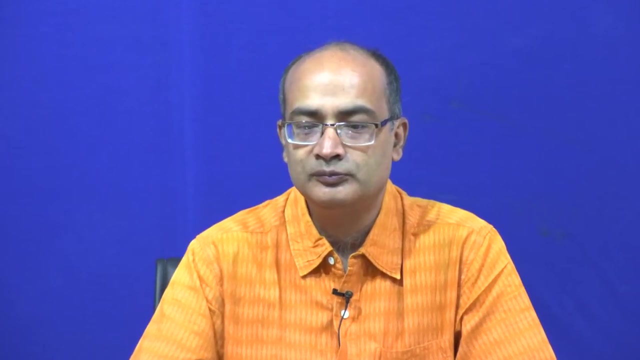 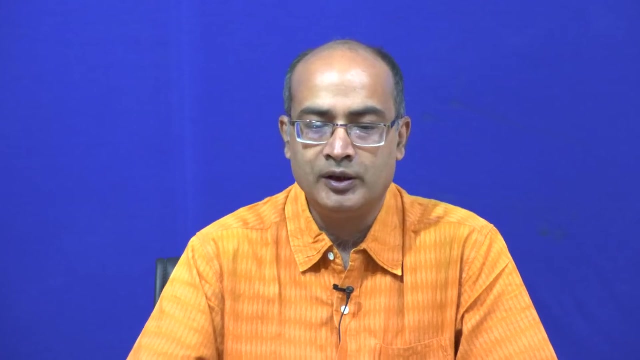 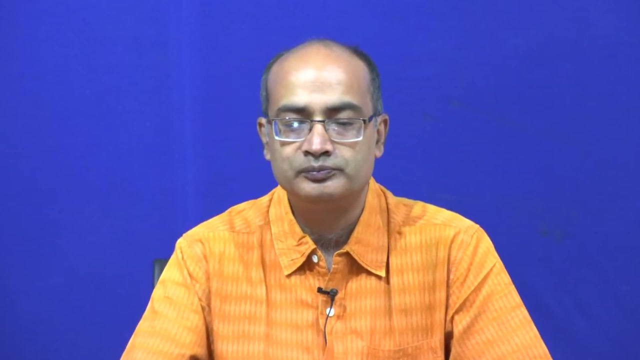 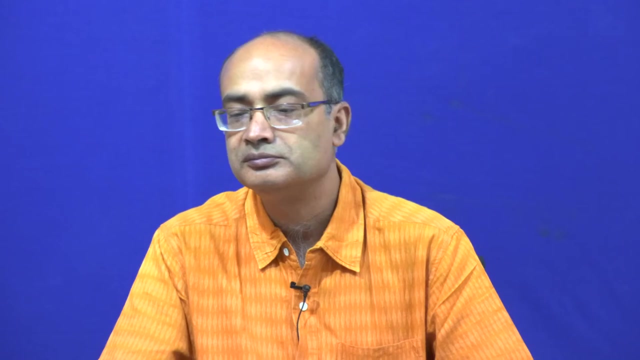 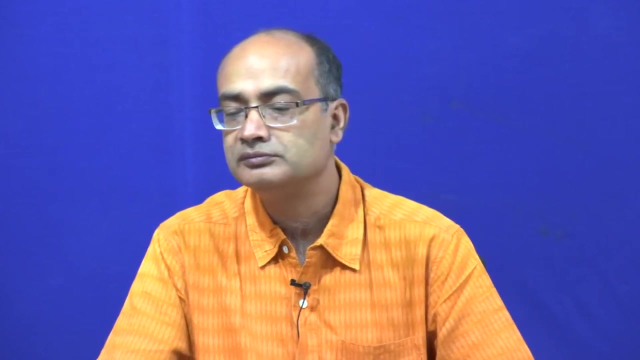 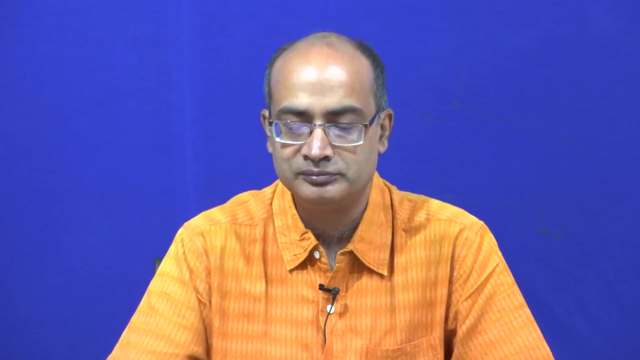 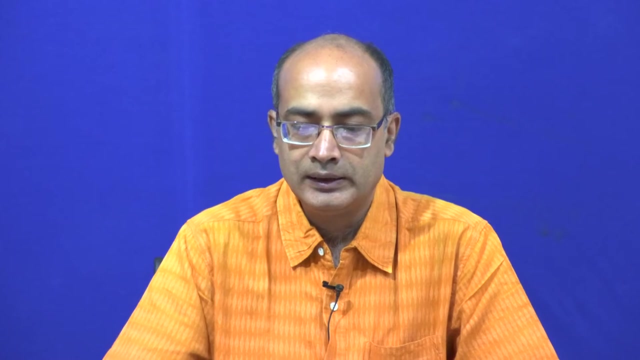 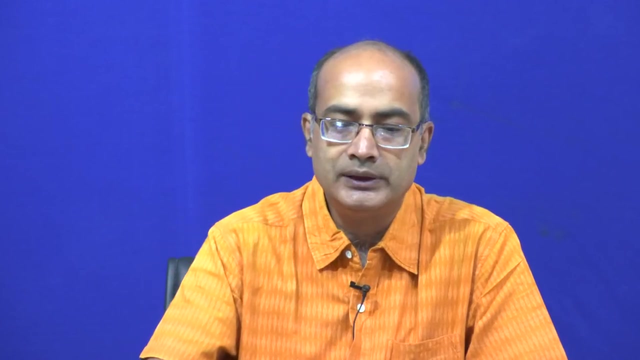 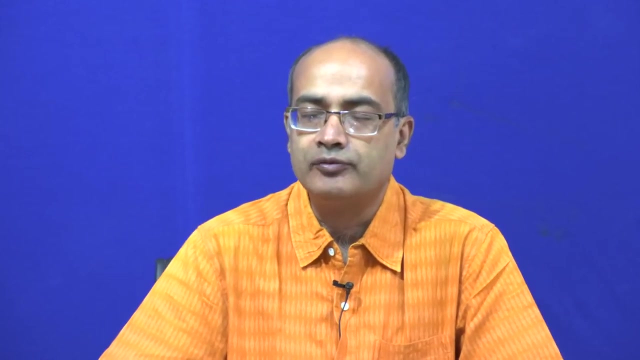 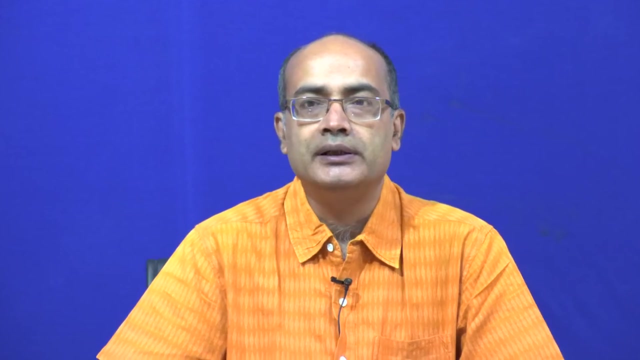 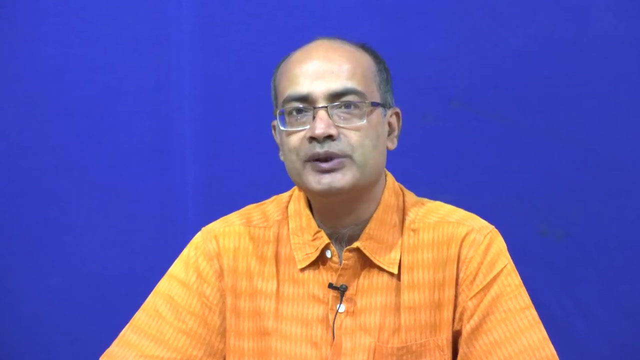 Thank you. Thank you. Regarding the the exam, I we can actually ah take some of the that points that, first of all, in the exam, that what I get, that there would not be, that MATLAB will not be available, So that there are few questions based on MATLAB and primarily they are introduced. so 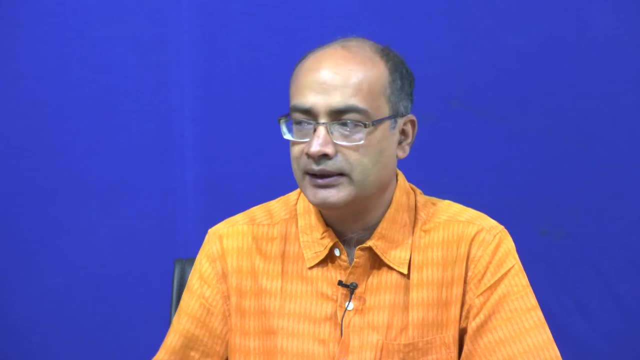 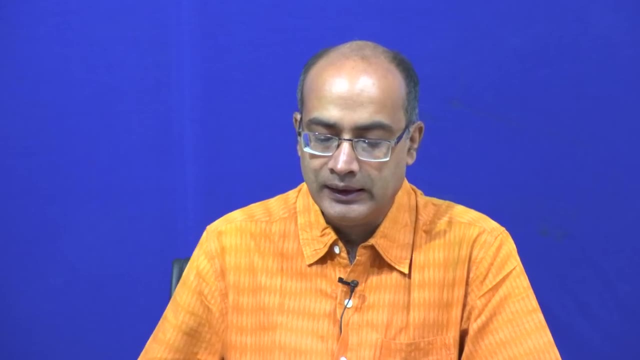 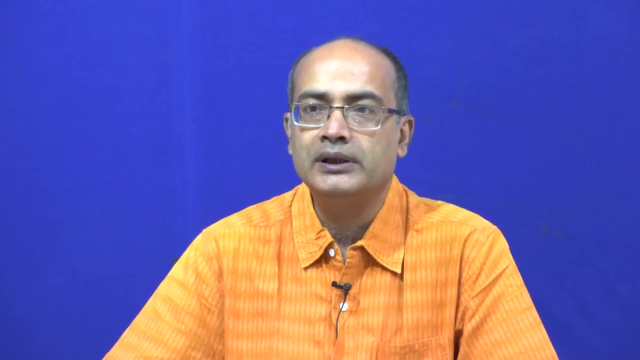 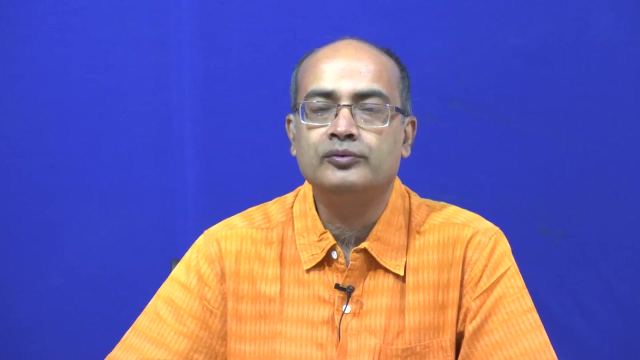 that you can appreciate the the text in a better way. Those questions, That that those questions actually we would not be able to ask you in the exam, simply because that the MATLAB support will not be there, ah, at the time of the exam. ok, will not have access to the MATLAB. 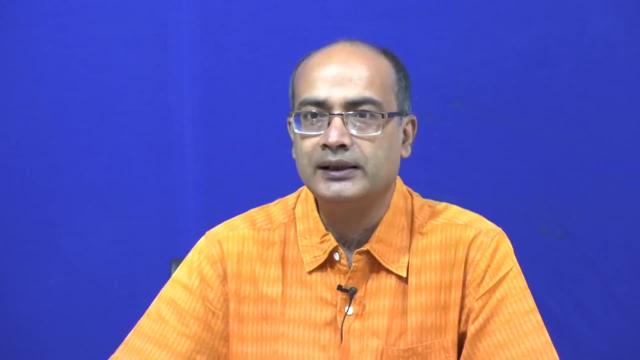 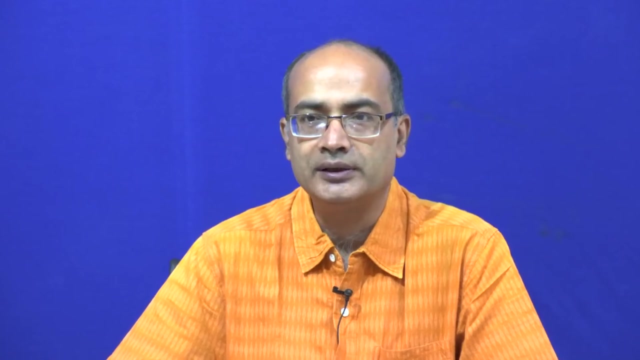 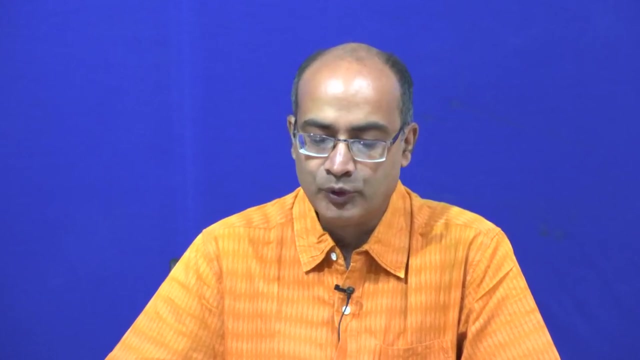 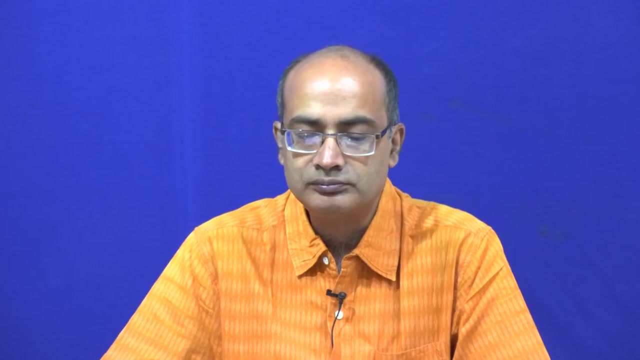 So those kind of questions would not be there. However, the keeping that in mind, if there is any small computation, you keep them small so that you can do those computation using calculator if you know the equations. ok, We got one more questions, so let us take that before we come back again to the exam. 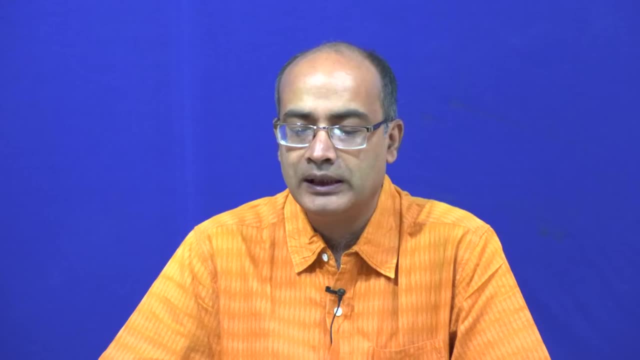 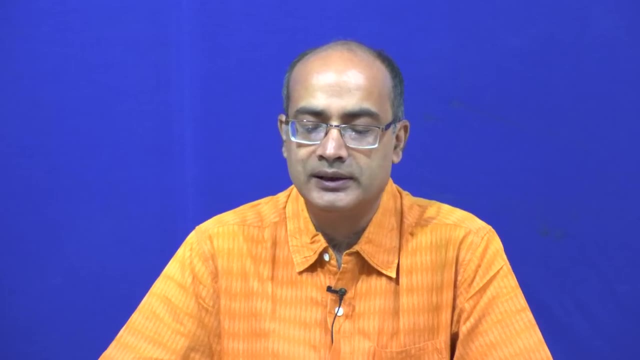 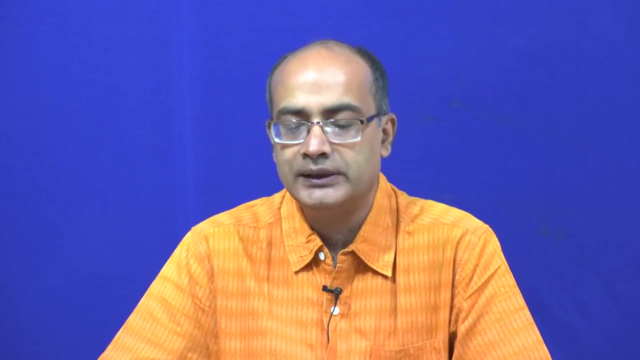 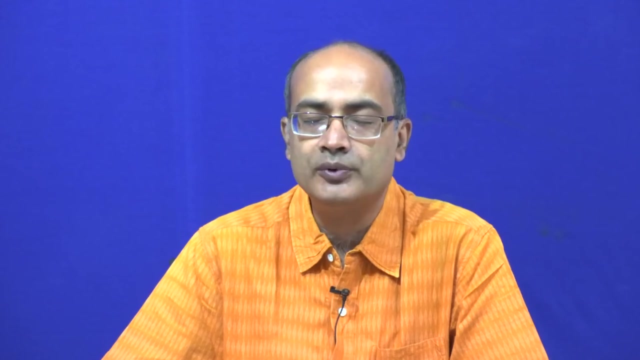 How to understand mathematical equation for biomedical signals. This question, for came from Pankaj Kesari. it is a very good question, Pankaj, that when we actually teach actually biomedical signal processing we try to go step by step to explain you that. What are the assumptions taken? 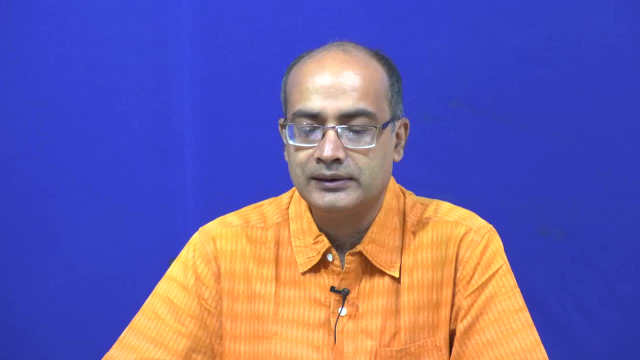 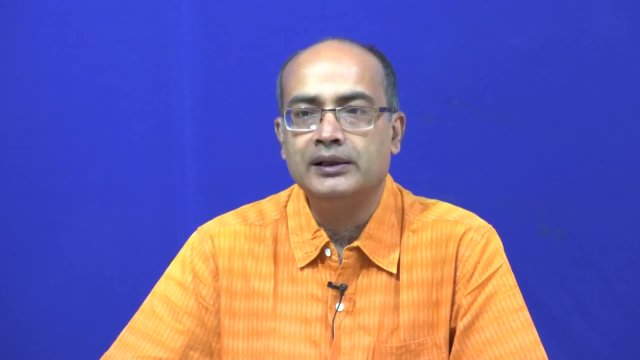 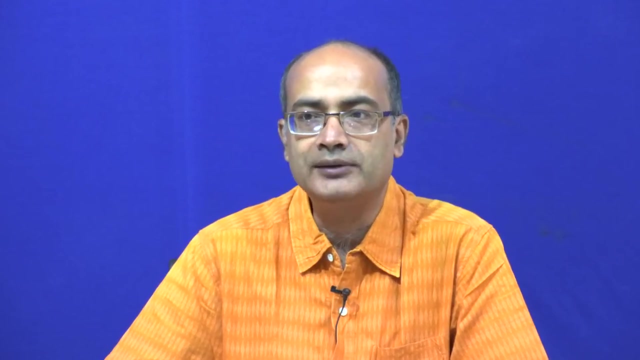 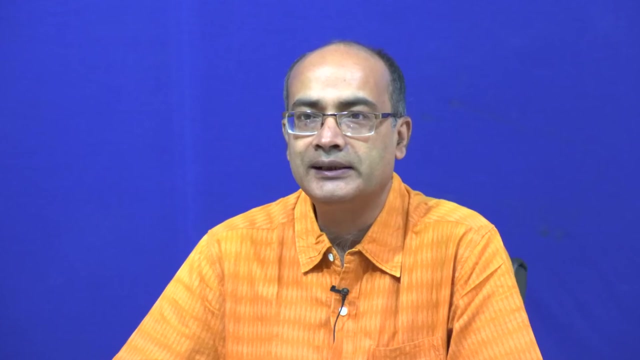 For that and that the way you have to do that you need to take actually those equations and try to derive it yourself and whenever you will fail, then if you cannot do that, you should look back to the book or the notes to see that how the derivation is performed. 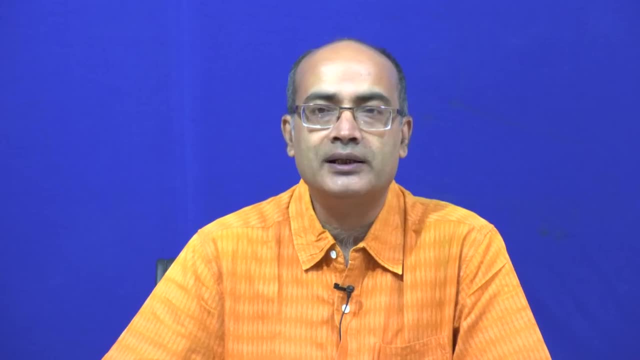 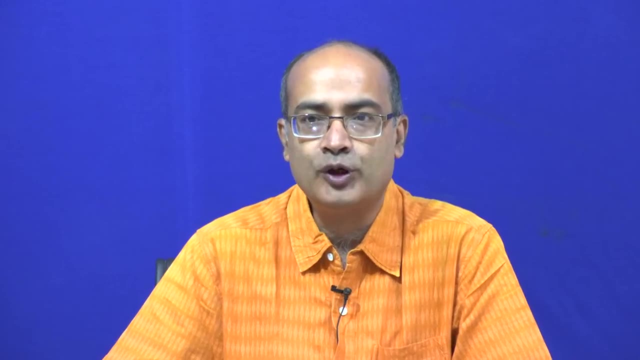 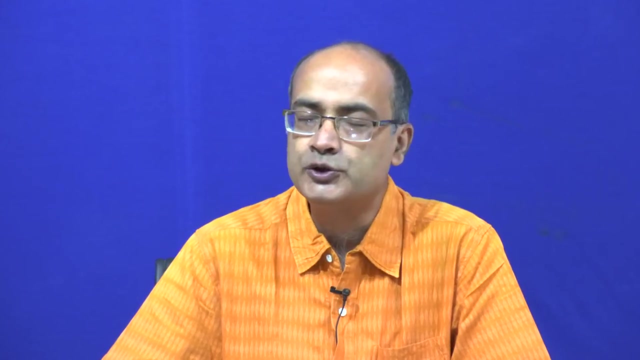 There are number of tricks that is applied Sometimes. Sometimes there are different formulas that is used. usually we provide them and sometimes it is from our, the basic: the knowledge of signal processing. So here what we assume, actually: that you have the knowledge of signals and systems. 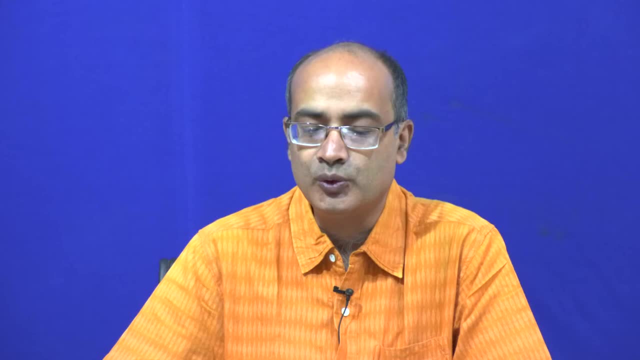 there is a must that you should have that to take this course. and if you have that background, I think that you should have that background. I think that you should have that background. Ok, So you will get that. it is not difficult to go through them. 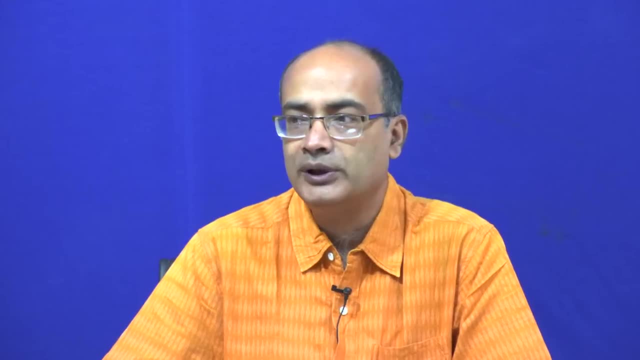 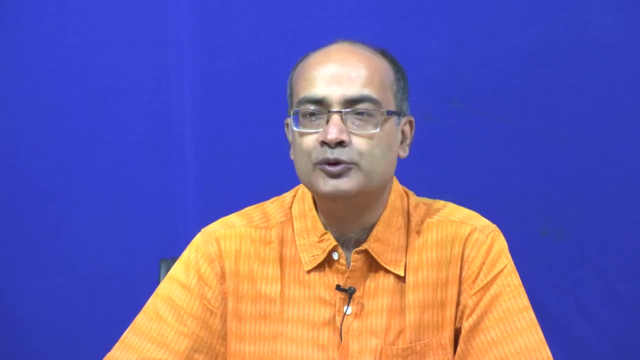 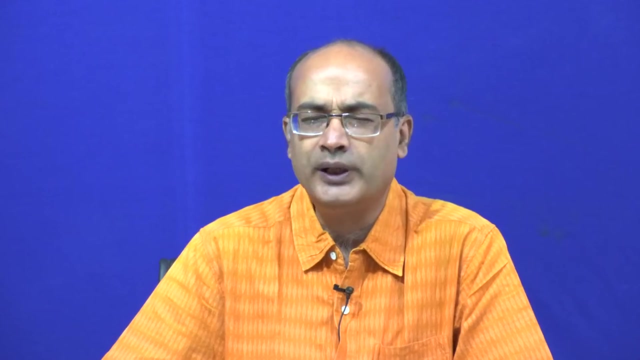 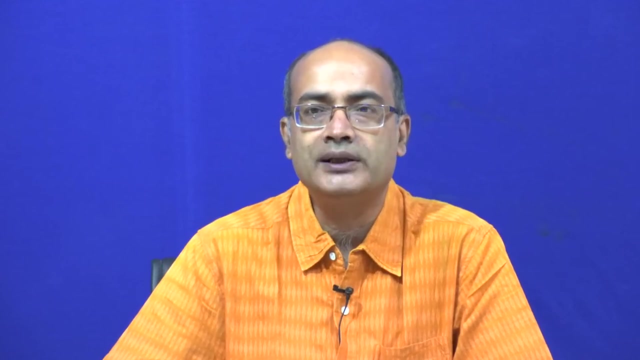 The only thing you need to patiently go through them line by line and you should try to derive them that line by line And there is no point trying to memorize them or mark up that. that is not required. you should appreciate that. what are the tricks played at different step to derive them? 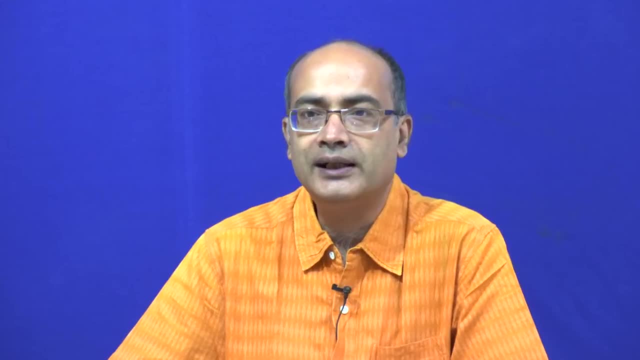 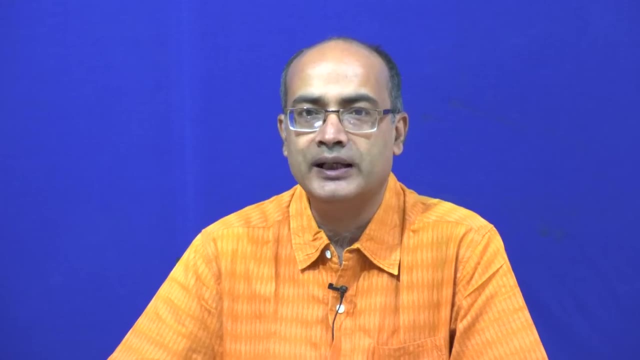 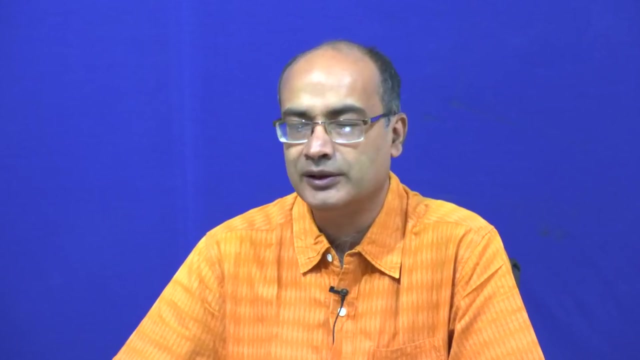 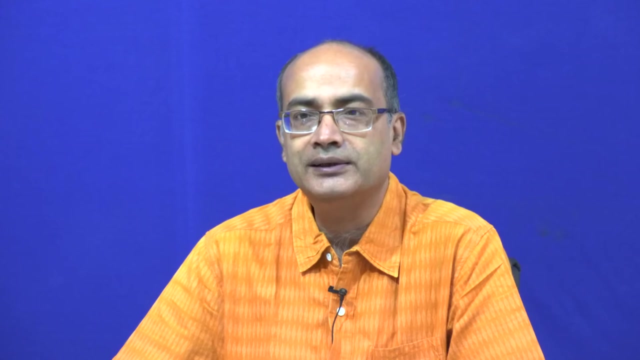 Ok Now, if you are a science student, to get the desired answer. So how the manipulations are done at every step, and the best way to do that, that you do those calculations line by line yourself. If you find it difficult, look at the book or the note. see that how they have done it. 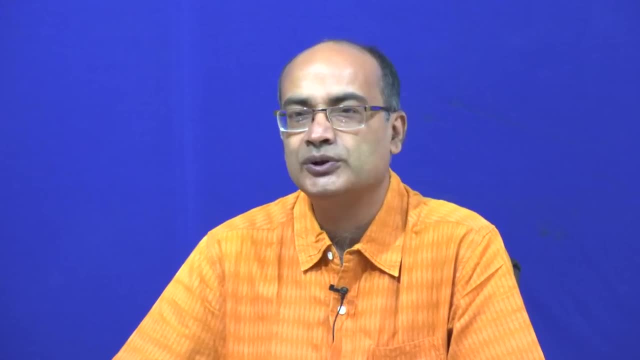 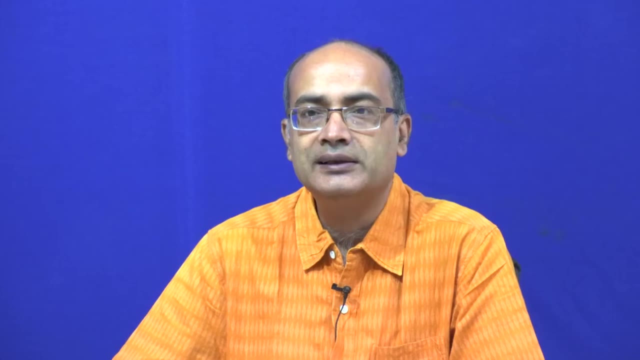 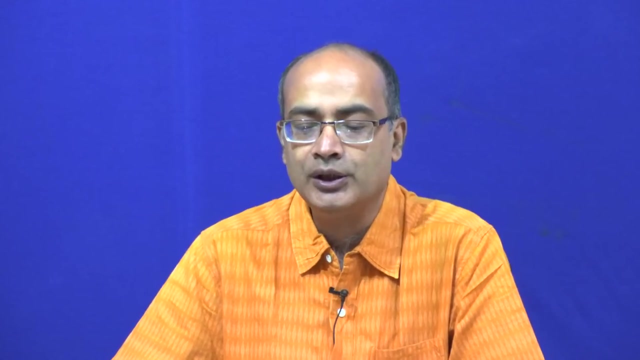 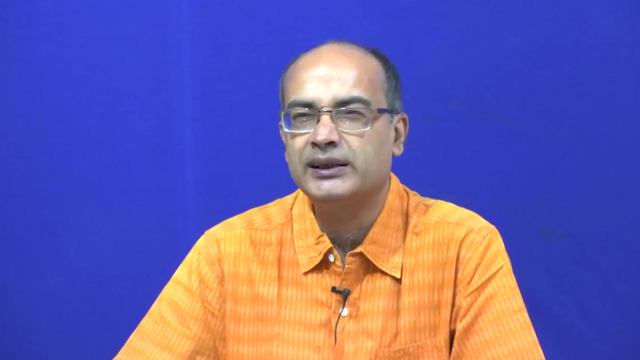 try to get that. what is the formula? they have used that to actually make that change or manipulation, and then how it proceeds. So that is the way to actually understand the mathematical equation for biomedical signals and, if you have some specific question regarding some derivation, that is are how you have gone. 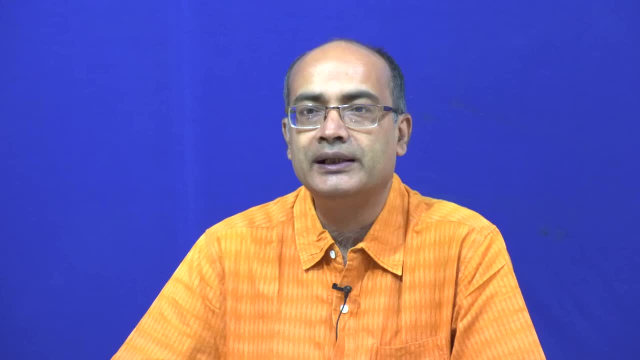 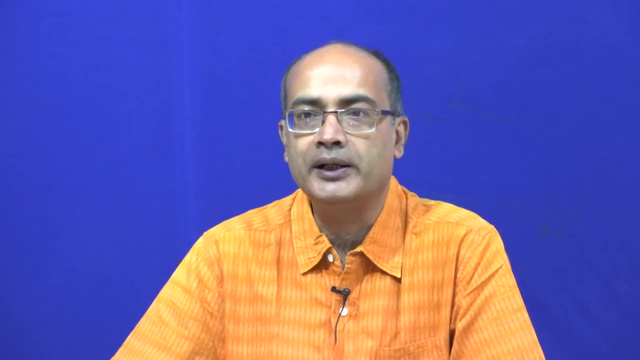 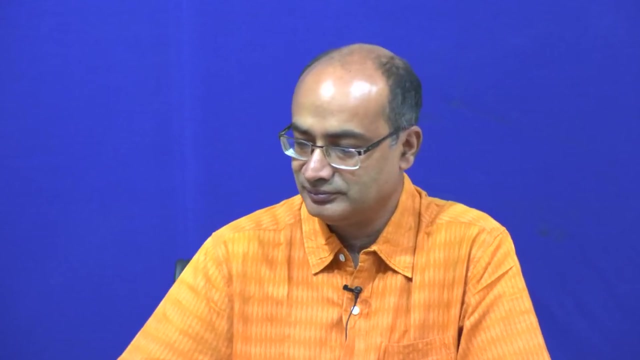 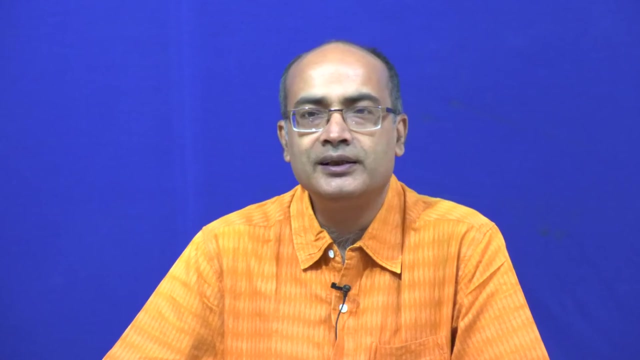 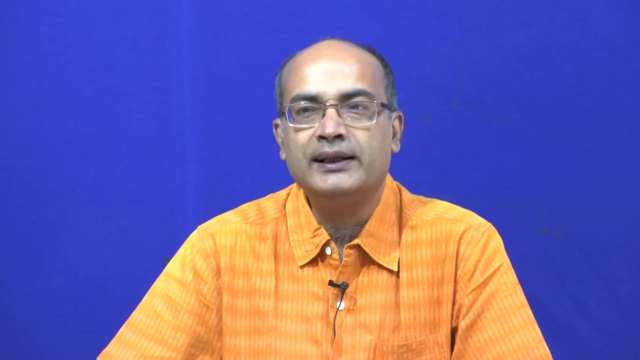 from line 1 to line 2.. So in that way, So you can make such pointed queries in the forum, we would certainly try to reply to you. So, going back to the that, the exam that we need to look at, that, the whole syllabus, that- 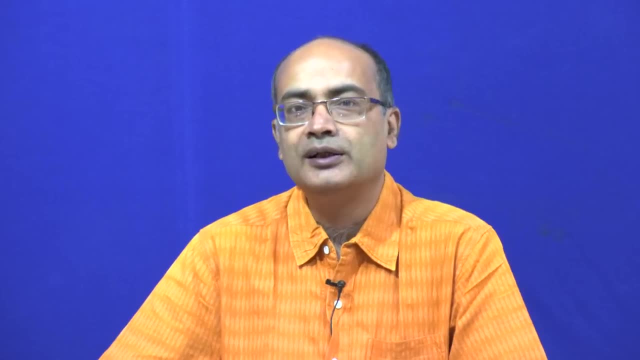 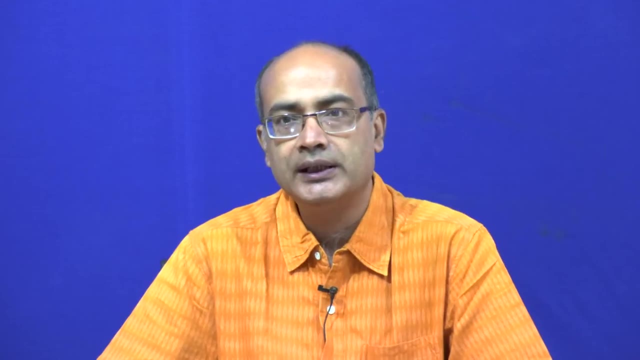 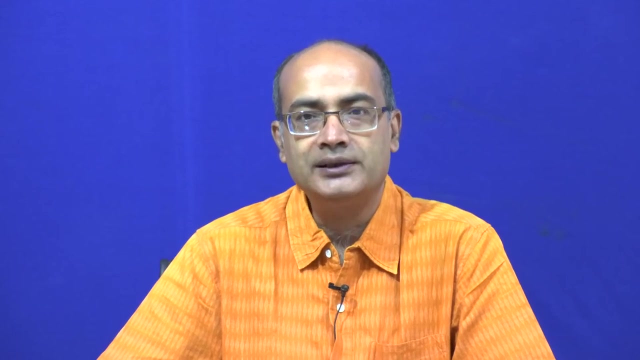 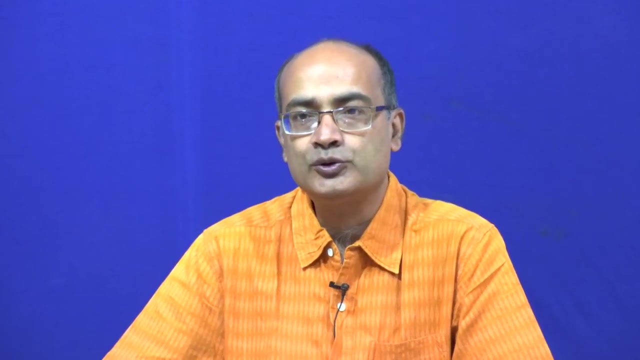 is. So that is one of the criteria to be prepared for this exam. In the first 8 weeks we have actually covered the whole syllabus and after that we are taking the tutorial So that you can appreciate those actually theory in a better way, and that also helps. 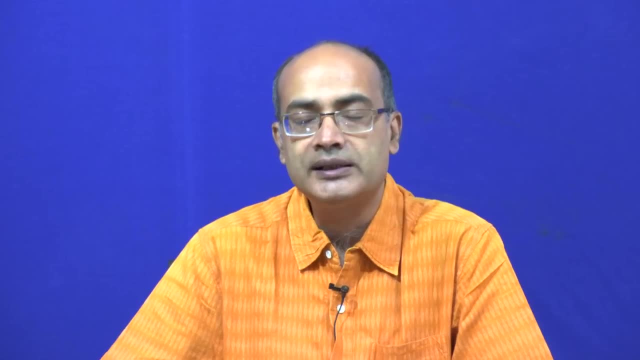 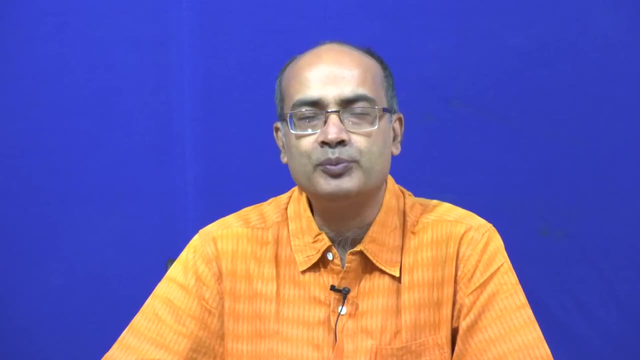 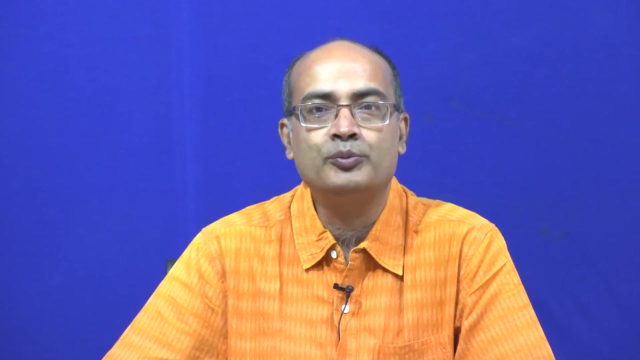 you to get acquainted to the real signals. Otherwise, after taking that course, if you do not know how the carotid pulse signal looks like or how the ACG signal looks like, then I think that we have not been really successful in teaching you. So you would get the introduction about that. you would know that. what are the specifics? 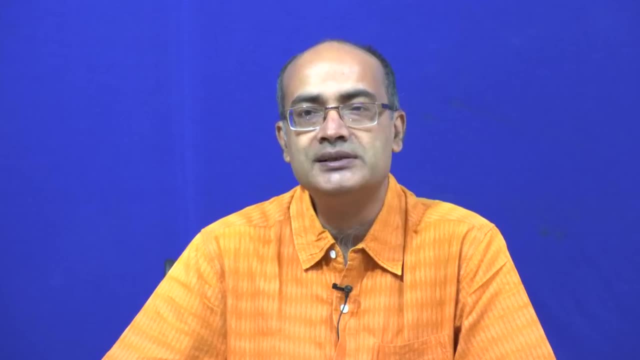 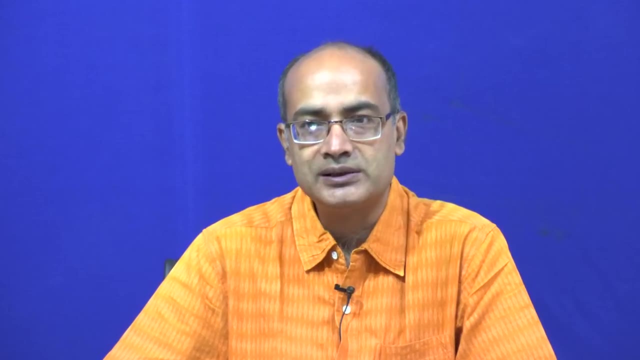 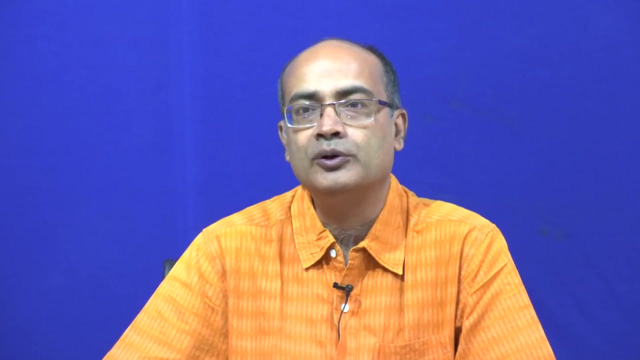 of that different kind of signals and at the same time you have a brush up of that, the, that, the syllabus which we have taken in the first 8 weeks. So you have gone through that, you have covered through the whole syllabus and I think you 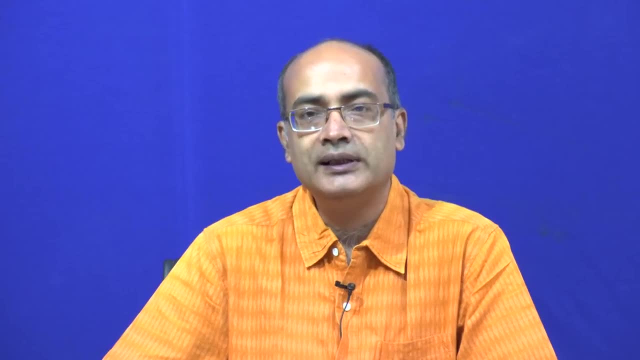 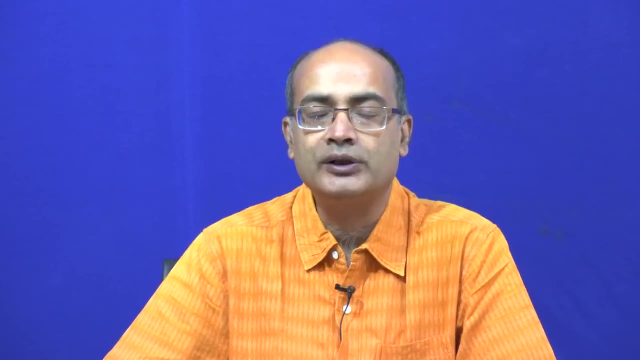 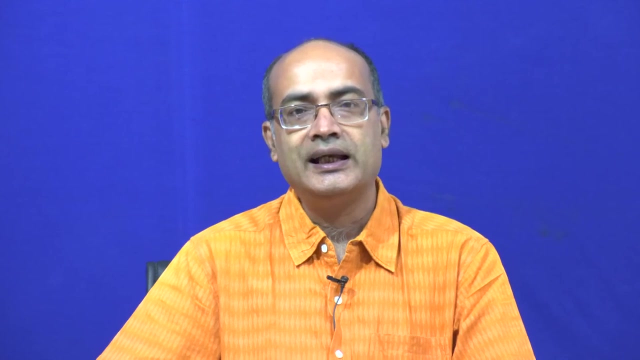 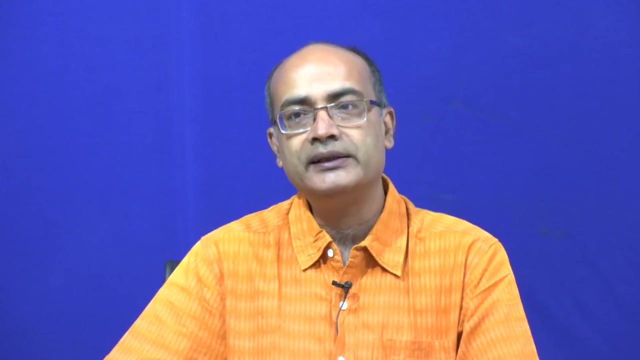 have also participated in answering the assignments of that, So that itself is a good practice actually for the exam. So in the exam you would get very similar kind of questions, may be a little deeper, because over the time you are expected to have more insight into that subject. 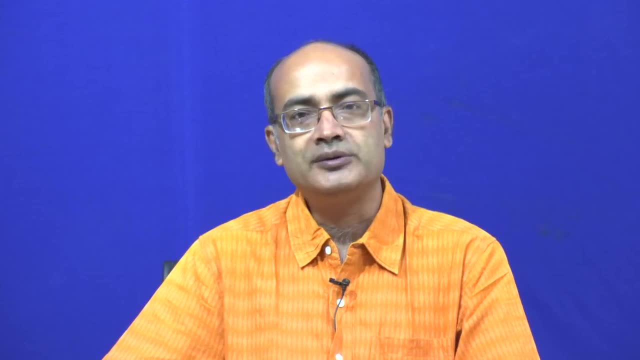 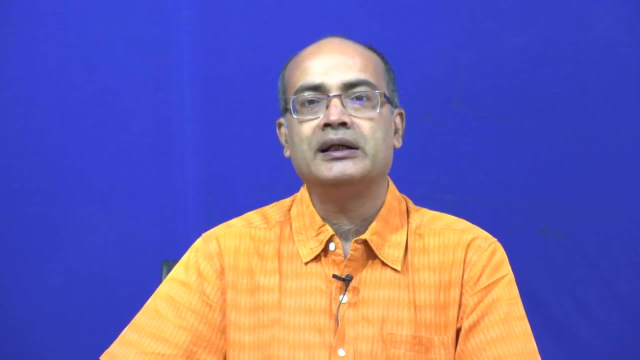 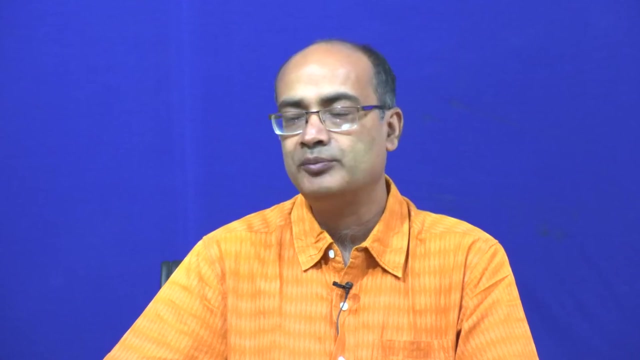 So few questions should be there which would be just like that. that assignment- very easy, Some of them if you just read through that course or just listen to the course, even you are unable to understand. So you should be able to do the assignments, you should be able to answer. 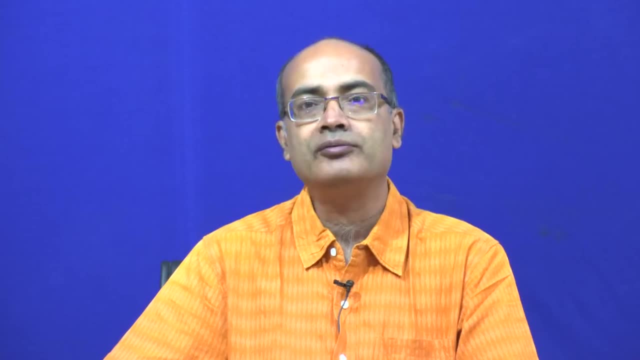 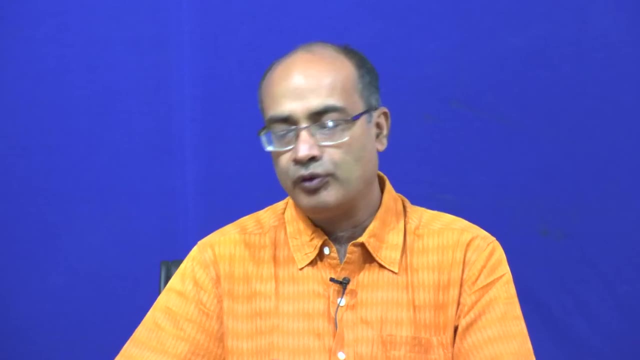 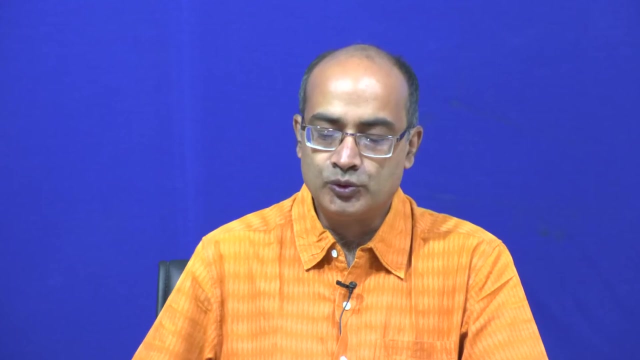 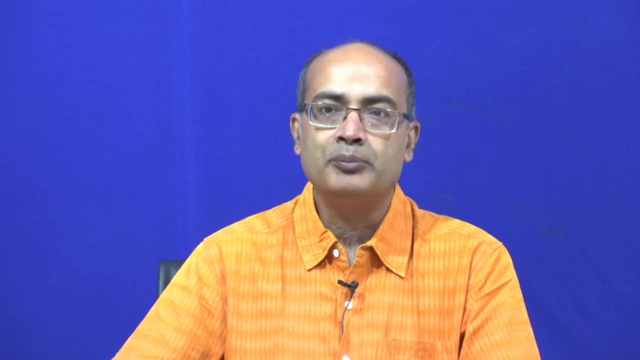 For few questions to answer. you need to have that practice of actually writing those assignments and for few of them you need to learn a little more, you need to go through the books and to get a little more understanding. So primarily that the questions should be there. 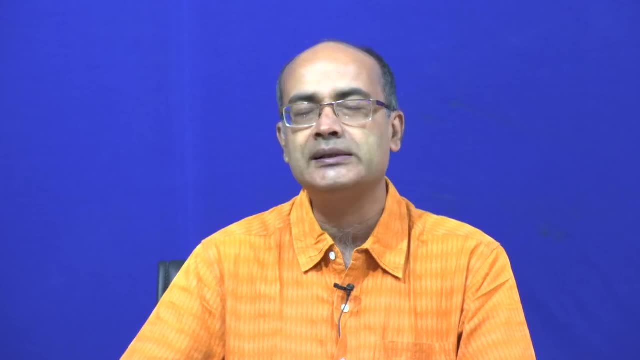 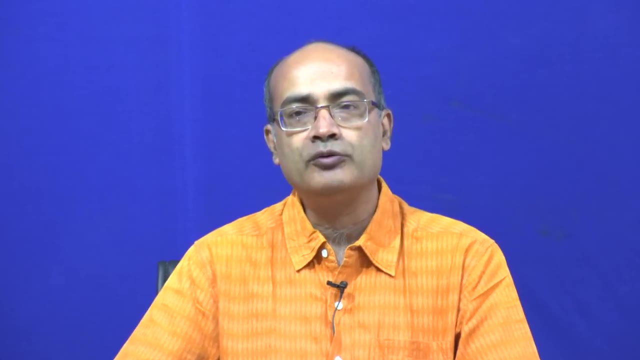 So you should be able to do the assignments. you should be able to answer. Some of the questions could be divided in the three categories in terms of difficulty, though all of them. there would be short questions there would be. each one of them would be of: 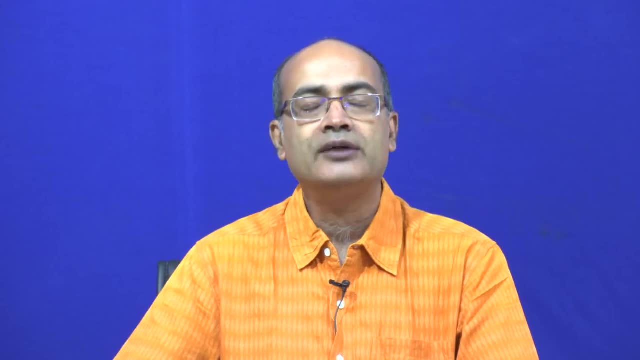 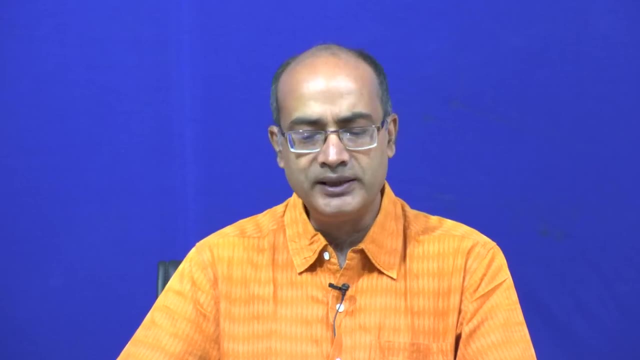 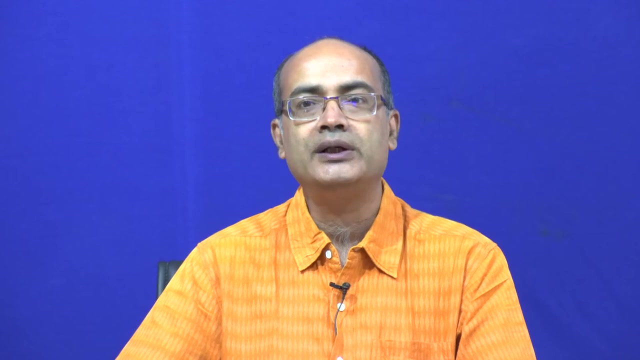 two marks of and you will get 50 such questions, so that you get 100 marks to answer within that time. So we will have plenty of time because they are objective type actually questions and I do not think that you will have any difficulty in actually finishing that. 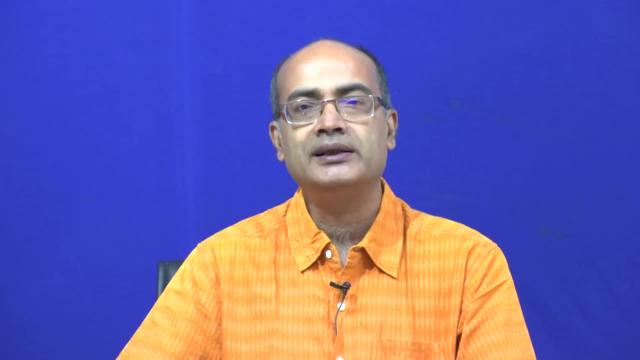 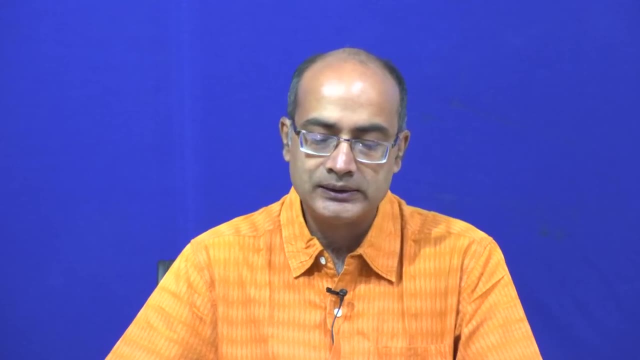 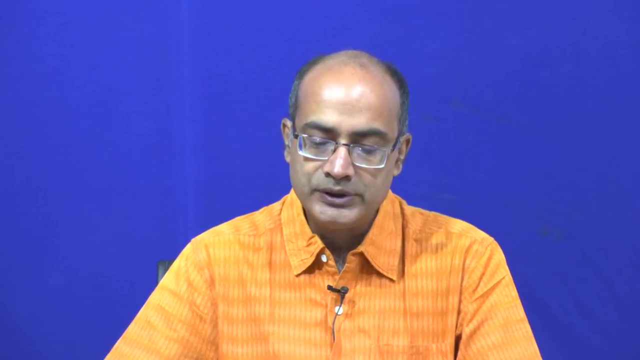 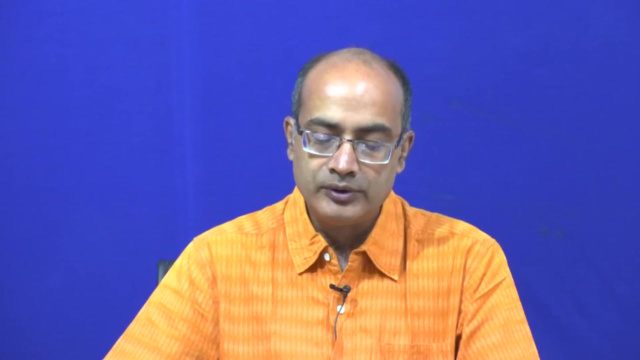 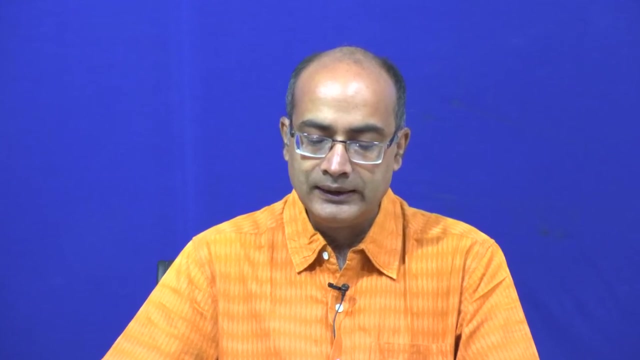 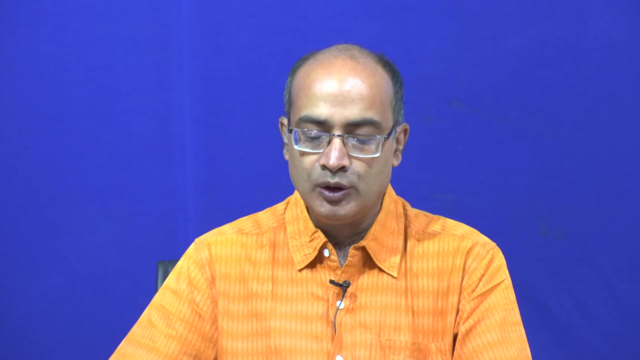 The question in time. we got one more question from Ashish Kumar Das- how the morphological characteristics are used to use as a feature and classification of ECG signal. that in case of ECG signal That We look at, that, the different kind of characteristics, for example, that the first thing, what we look. 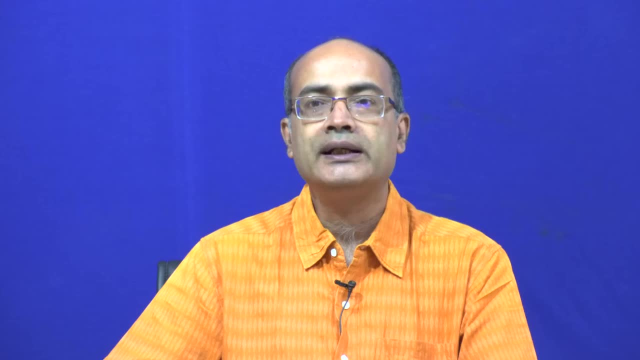 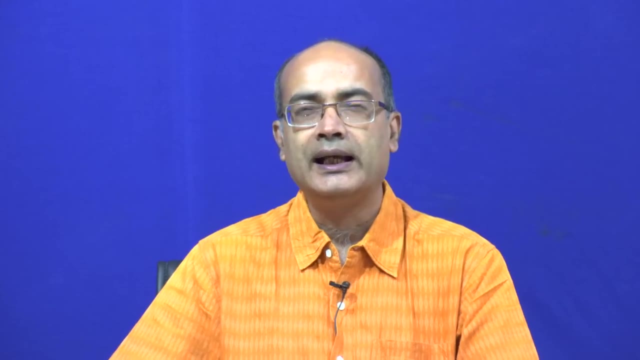 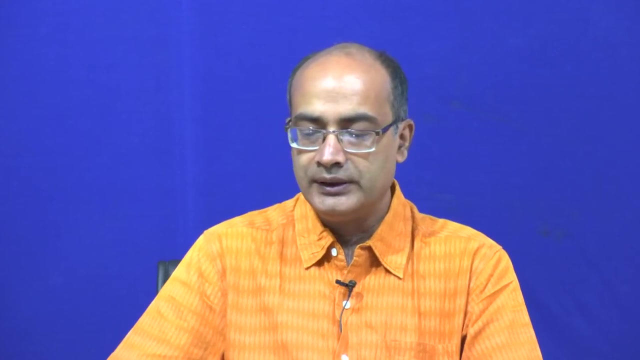 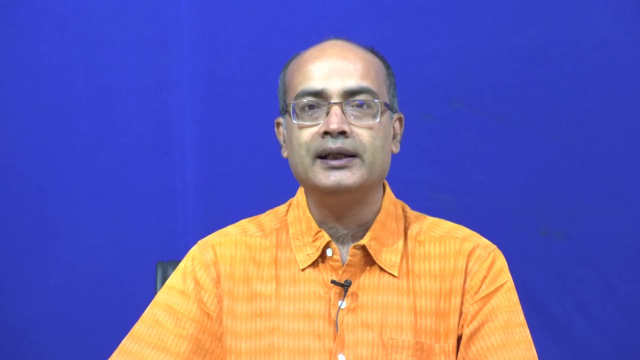 at that. what is the rate at which we are getting the ECG signal For that? we look at that when the beats are arriving and the interval between two beats, which we call as RR interval, We actually take that. So that is the first signature for the ECG. 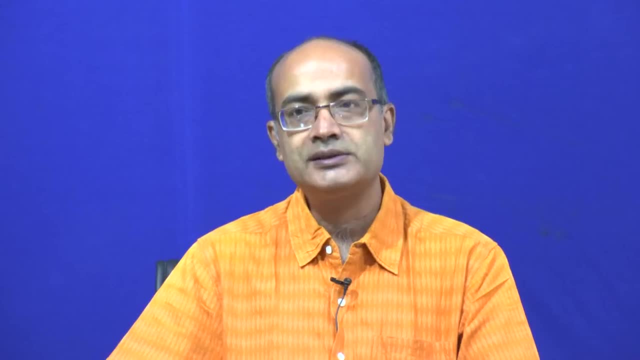 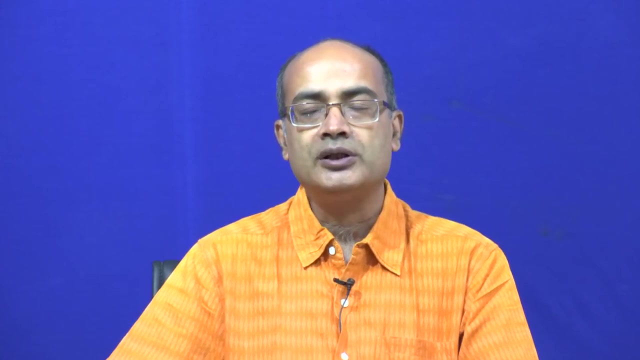 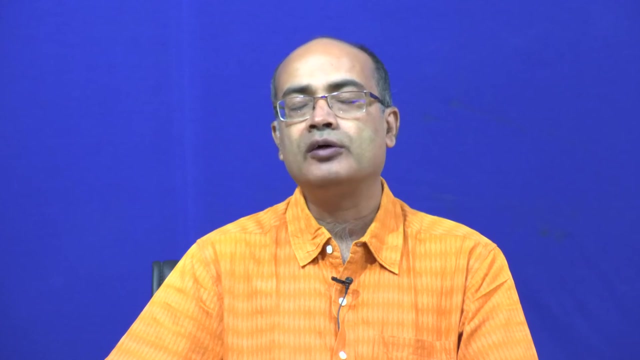 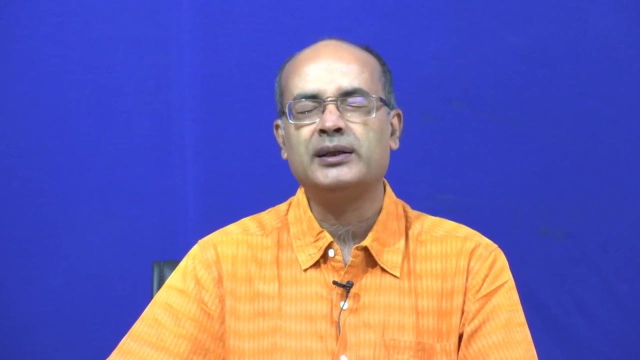 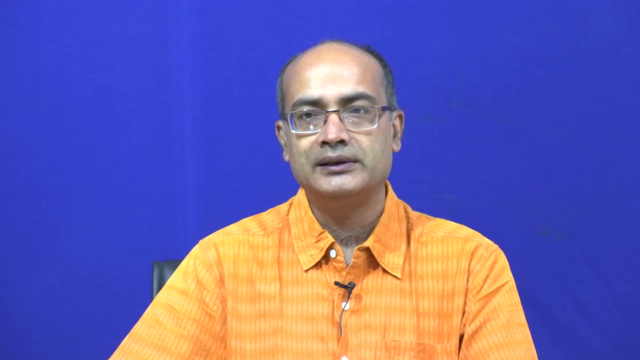 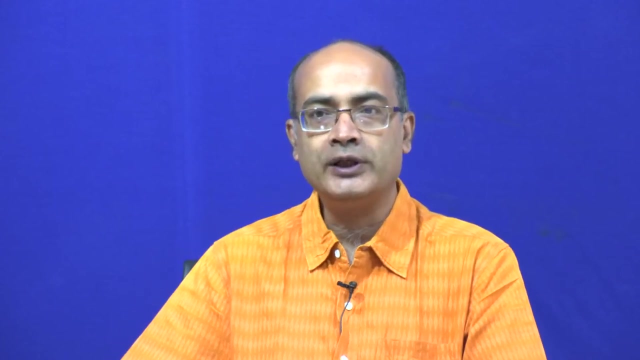 Then we look at that. other characteristics. you know that the people have tried correlation. that is one. then, due to ectopic beat, that the QRS complex may be jagged because of say that, So in a different way, rather than trying to take that as a shape, we have derived it. 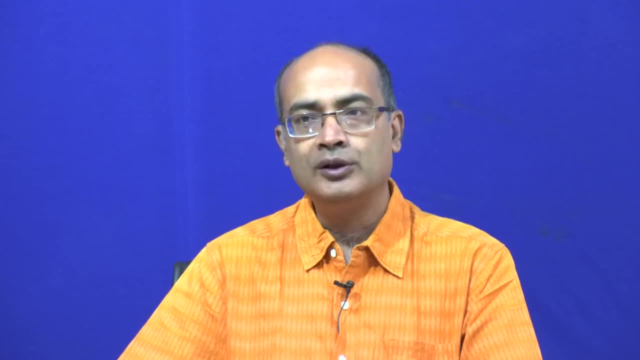 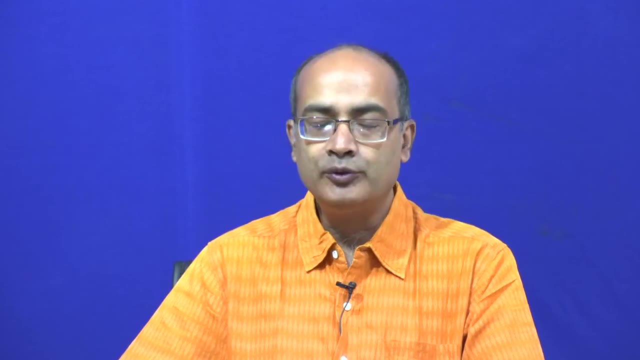 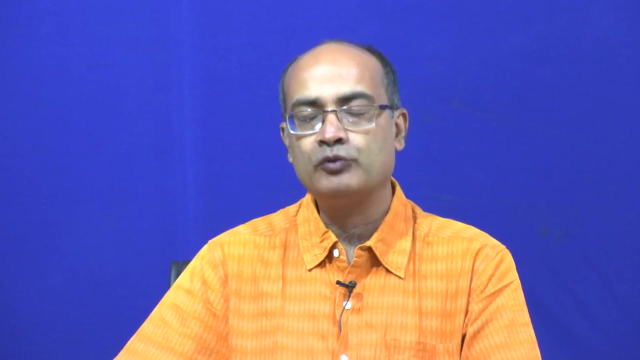 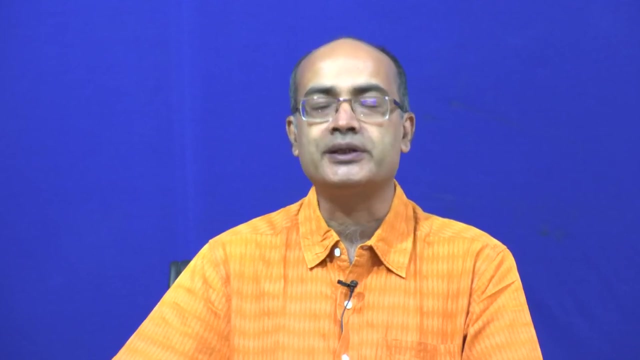 as a lump parameter when we have taken the signal length. So, in different way actually, we have actually taken those morphological changes or captured those morphological changes in terms of feature to get that, whether this actually signal, Actually signal is coming from a normal subject or it is coming from a person who is a patient. 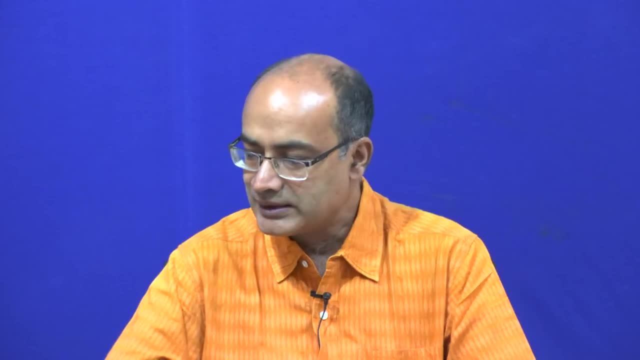 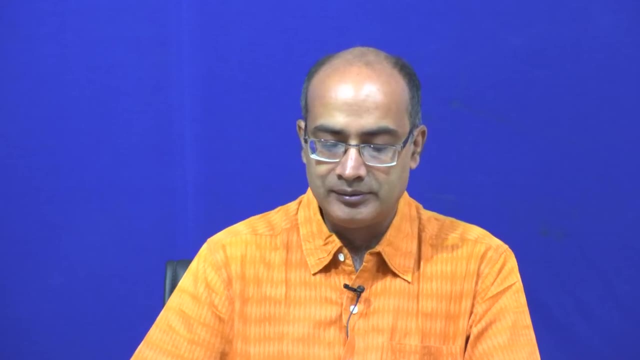 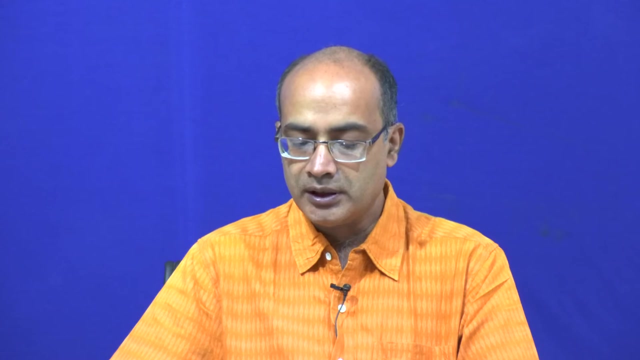 ok, So that is the way we can do it. this is just an example, But if you have some particular difficulty in mind, that we can actually look at that. The next question is from Lalith Arjun Kher. Why are not medical devices developed? 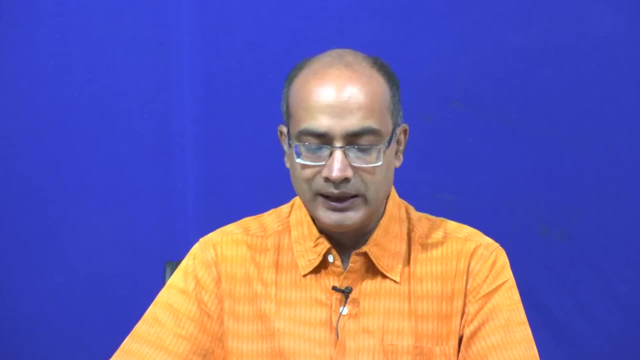 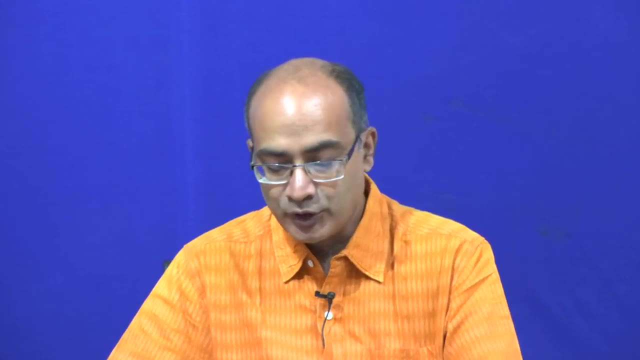 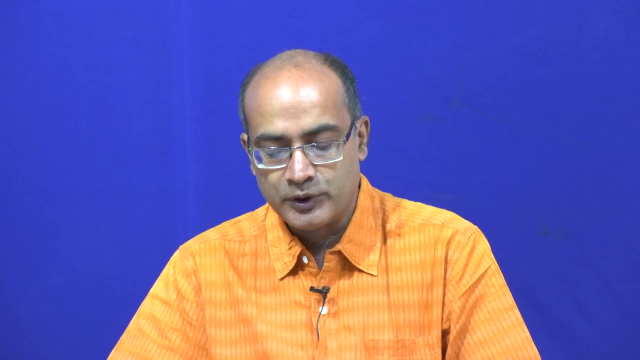 Why are not medical devices developed and made in India, despite good R and D in IITs? Lalith, thanks for your compliment that IITs are doing good research. I think it is not. the just responsibility is not restricted to the IITs. 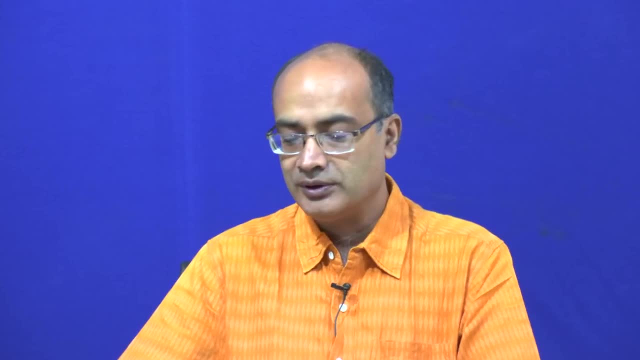 IIT is actually some institute. they are named as IITs.